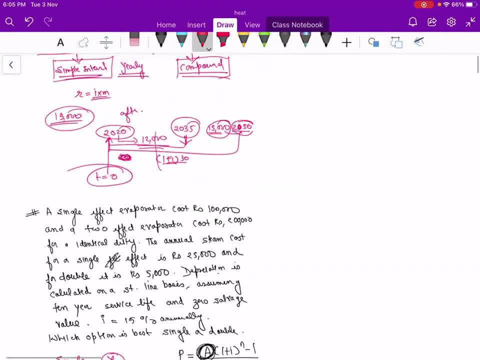 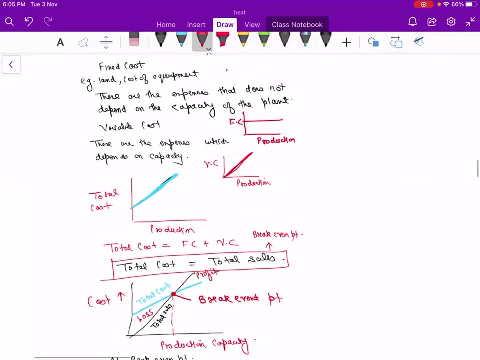 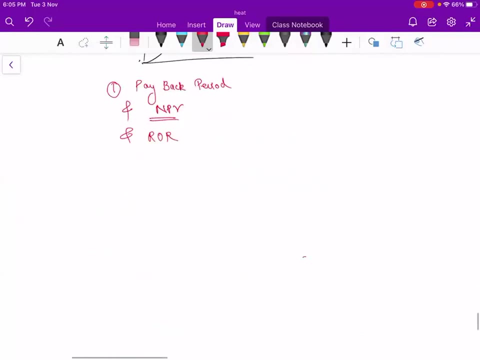 so that is the thing, and just some basic points, if you remember. So it will surely help you while solving this, all the things. Okay, so this much we have seen up till now. Okay, so we are now back to our position, that is, payback period, NPV and ROR. So basically, 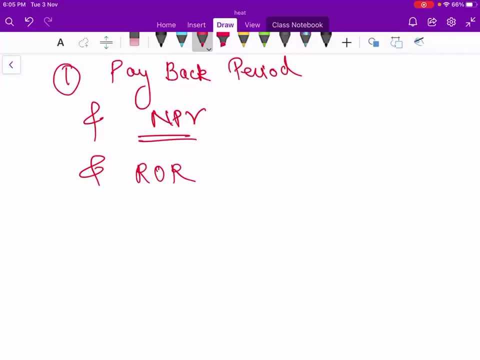 these all are profitability analysis method. Okay, we can say that profitability analysis method. So in this case we have GATE analysis that basically we can say annual rate of return, okay. okay, we can say npv, we can say capitalized cost, okay. 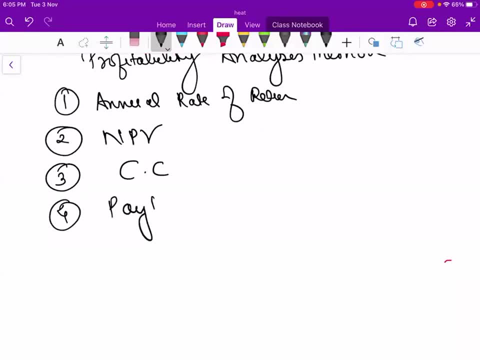 fourth, we can say payback period. okay, so this much we can say is very useful for our system. okay, uh, net present work, that is npv and other- is known as discounted cash flow. discounted cash flow, so it is nothing, but i effective. okay, just like i said, i will say: 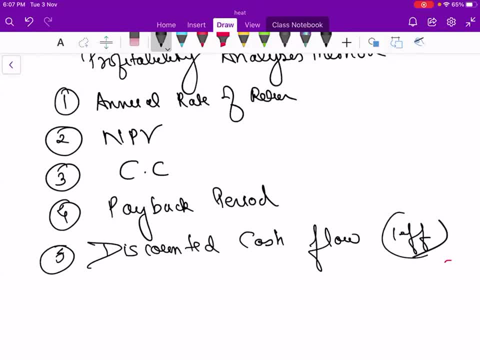 discounted cash flow. it is a another name of i effective, that is, discounted cash flow. so it is just given to confuse you. i will explain you. there is a one short difference between i effective and discounted cash flow. in value it will be same. okay, the value will not. 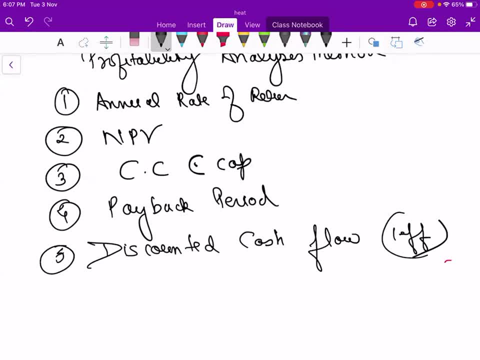 see: okay, cc is capitalized cost, okay, capitalized cost, and pv is net present value- okay. so these are the things so we want always that our annual rate of return should be high, okay, npv should be high, okay, capitalized cost should be less. okay, payback period should be less, and 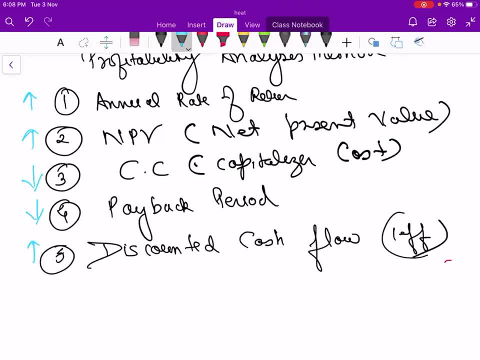 discounted cash flow should be high. okay, so you can uh, remember these arrows. actually. okay, because we want high rate of return. okay, we want net present value should be high. okay, that is present value. difference between present value and net present value: we will see. capitalized cost: we have seen. 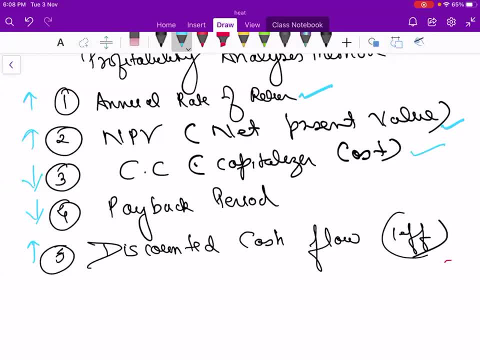 we have to select which is least one. so that should be low, payback period should be low. so we will today first see the payback period and cash flow. that is, i told i effective, so we know that i effective should be high. okay, so you can remember this. this is in the important. 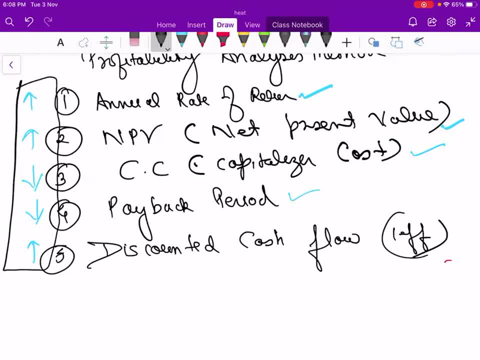 from interview point of view, okay, okay. so everyone got this point. what we are going to see is that we have to wait for this to happen and then we have to wait for the payback period. okay, so let's have a look at the scenario. so if we have a company and we are considering for the next 10 days. we have to wait for the next ten days, up to 10 days, up to 20 days, up to 20 days of the next day. then we should have to wait for the next 10 days to pay back a certain amount of. 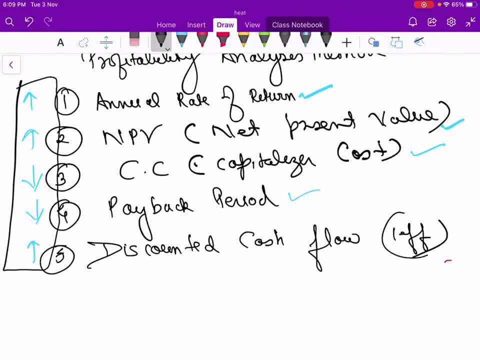 capital, because we know that if we don't pay back the first 10 days, it will then be canceled for the next 10 days. this is the annual rate of return. okay, everyone is comfortable, yes or no? yes or no, right in the chat section. fast, yes, okay, fine, so from this we have seen the capitalized cost only. okay, we have done with. 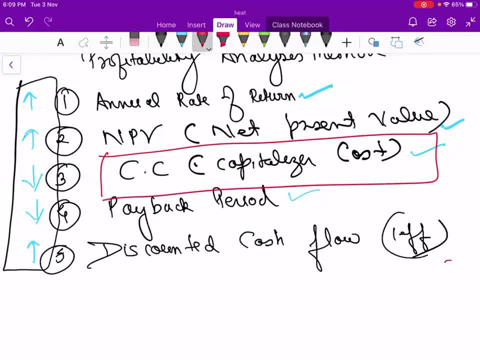 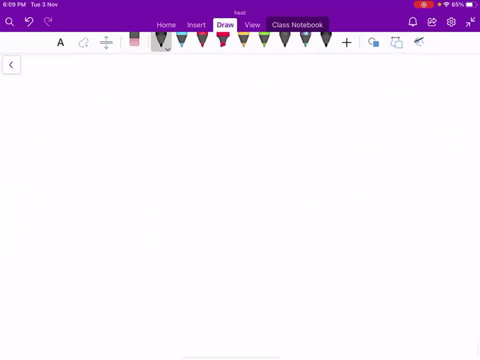 the capitalized cost. other topics we are going to see. okay, so first we are going to see payback period. so these definitions are basically you can say they are given by the economist because everyone in the world follows that definition. okay, so we have to stick to that definition. 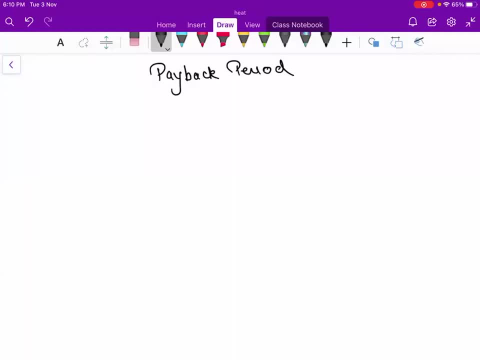 whatever it is told, uh the system means why depreciation is not for the industry, it is always for the other person. okay, so that way there are certain meanings of that. so payback period means basically means, suppose, uh, how much money you have invested. suppose you have invested 30 rupees, so what you will. 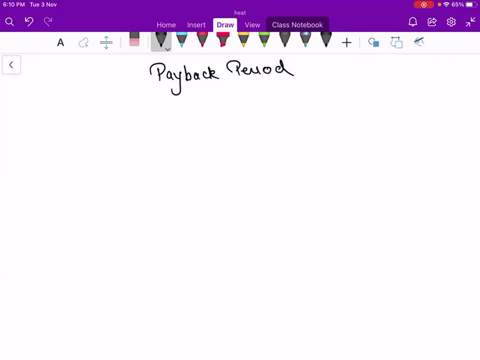 calculate that after how much time that 30 rupees will be? uh, get back to you. that is the time period. but in general, uh, meaning for us, for a common man, we say that if we have invested 30 rupees today, so from today we will count that number of days. but the economics say no, you don't have to count the duration of. 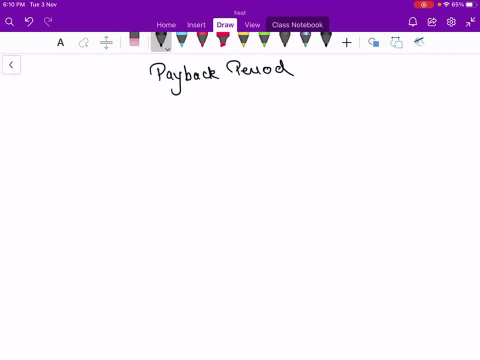 construction. it means that suppose you have invested 20 lakh crore rupees for any highway. okay, so in high, if highway is there, you know that in highway there is a toll tax. okay, that collect the money from you. okay, so that toll tax will start when that road operation will start. okay, it will not. 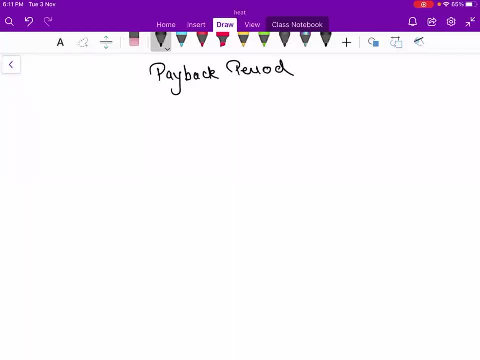 start from that day when your construction work is started. okay, we have to ignore the construction time while calculating the payback period. okay, so, basically, payback period means when the operation will start. from that day we have to, uh, count our payback period. so, if i draw a, 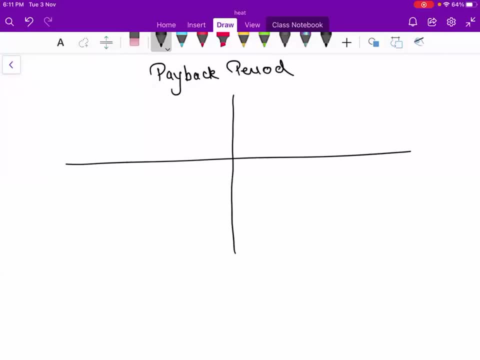 it is not up to mark graph, okay, so don't go on that. just see the axis. okay, don't go about that. how much it is going down and how it is going down. so if you want to start a chemical industry, we will be talking about the chemical industry. what you will do, we will do: first, purchase a land. 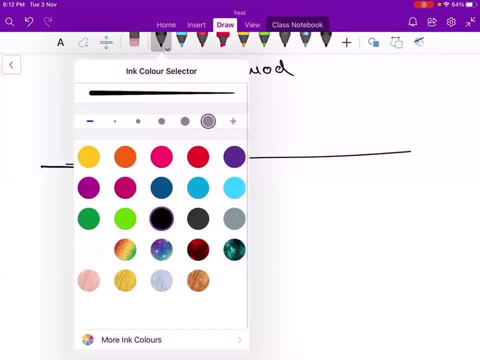 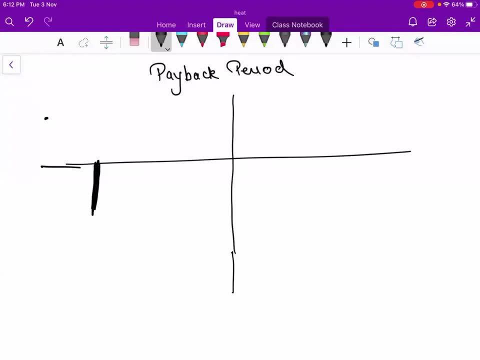 okay, we will first purchase a land. we will first purchase a land from there. so it will be sudden. okay, so you can say: buying land after that, what you will do, you will purchase the equipments. okay, so this equipment line will go like this: equipments, then here. what you will do, you just will reach here. it will be again sudden. drop this. 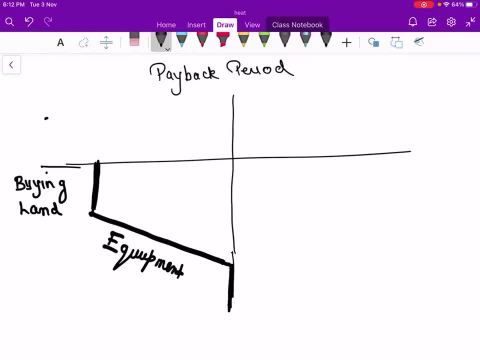 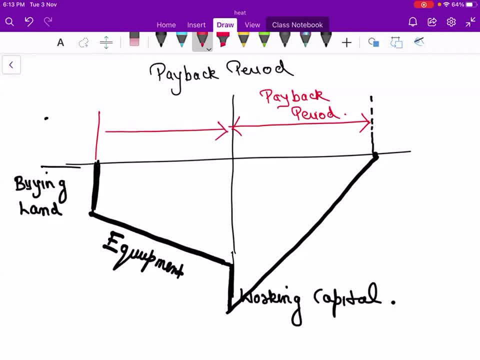 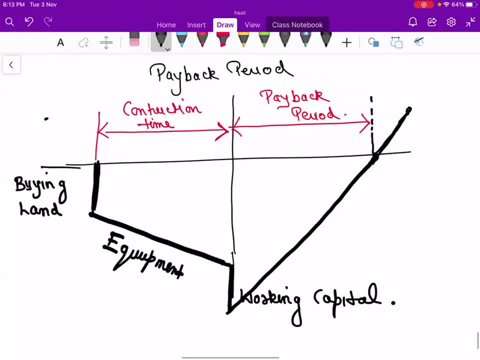 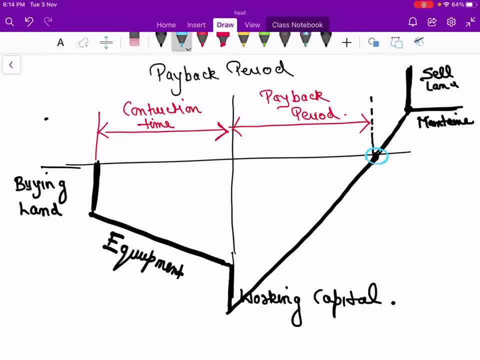 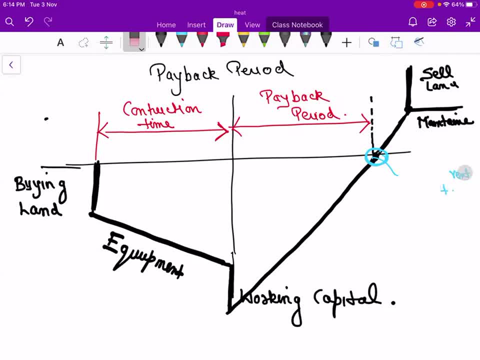 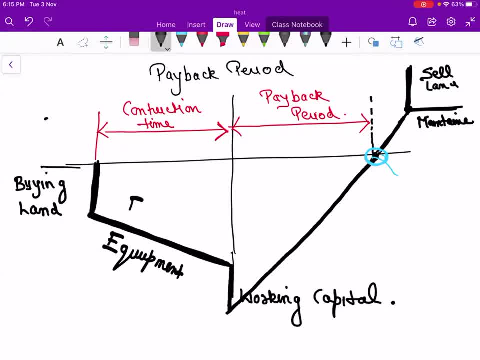 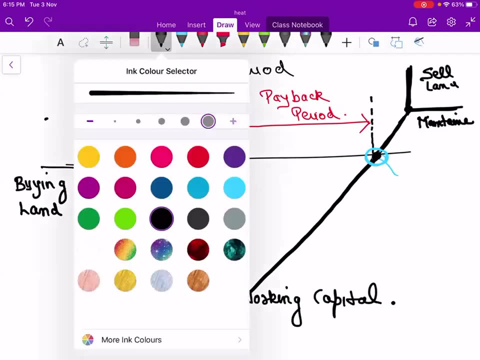 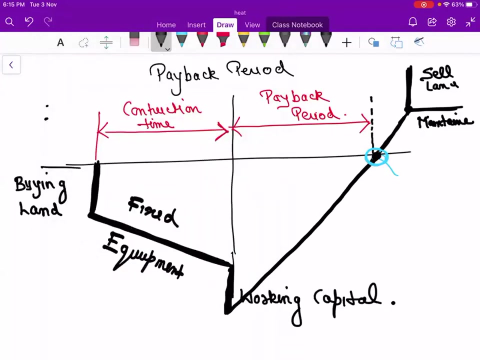 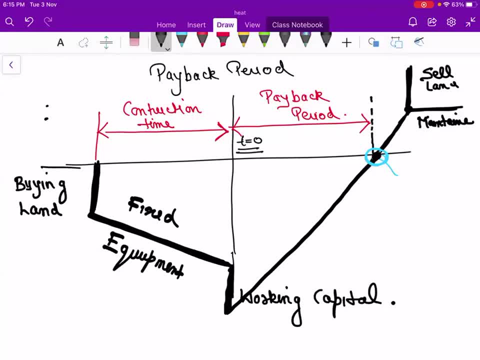 this is the point. this is the point. Time t equals to zero up to the point where it will intersect. So here, see here, the slant line is only recovered means only fixed capital is recovered, Working capital you have not recovered. For recovering the working capital, it will be recovered at the end. 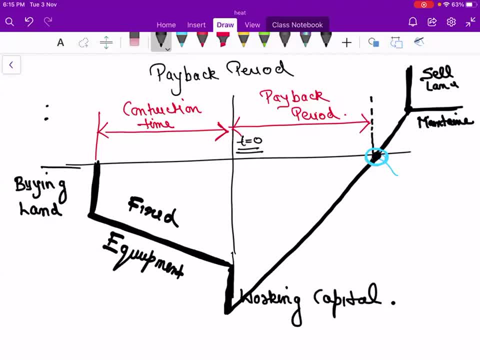 We will be recovering only fixed capital. It means that take back period is the time to reach the point after commissioning of a plant. it includes only fixed capital. It includes only fixed capital investment, In that working capital is not included, as well as construction time is not included. 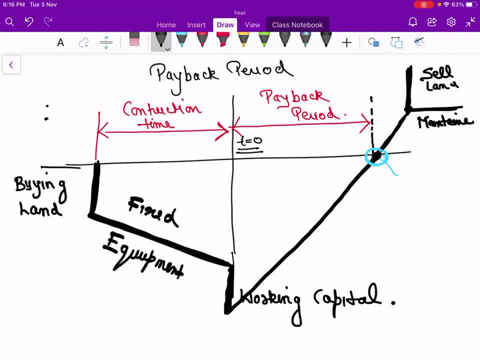 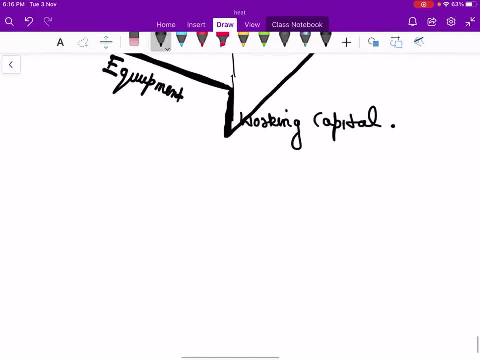 there In so many books it is given wrong. actually they have included the construction time also. So remember these points here. Specifically remember these points that construction time is not included in PB. PB is payback period. Second point: working capital is not included. 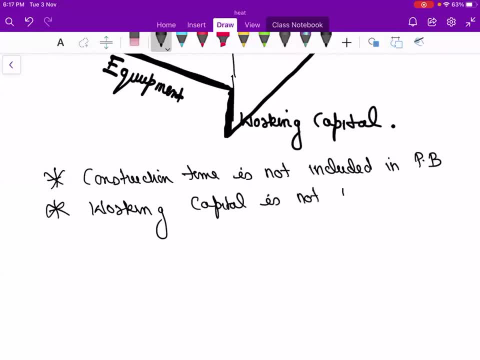 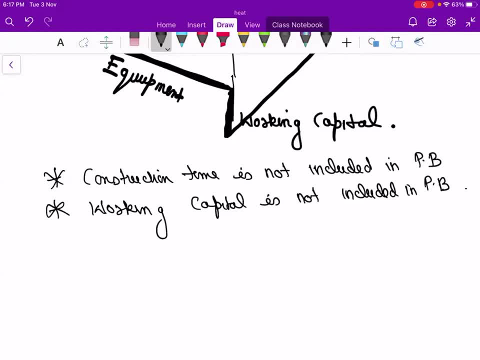 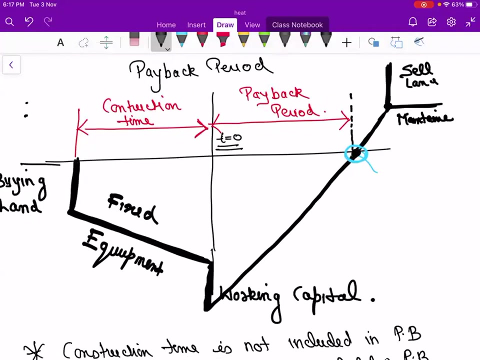 Software in PB. Okay, These two points You have to remember. Okay, these two points you have to remember. Everyone got this point. The draw this I will explain once again. does draw this diagram, okay, and think on it. And one part: future BI can work. basically, that the 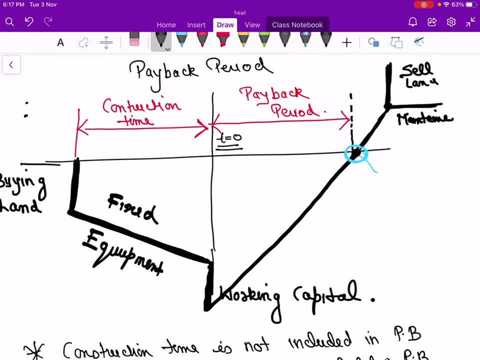 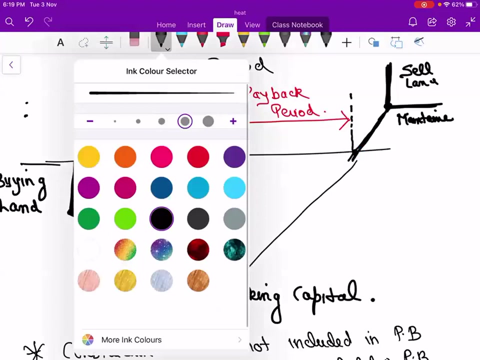 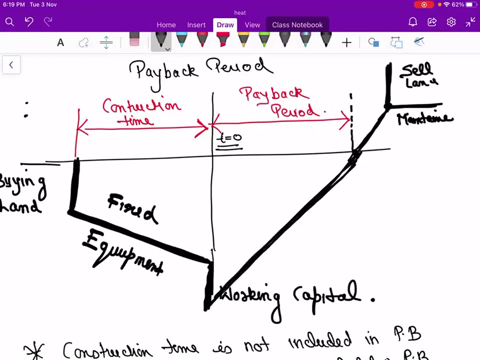 Okay, Everyone got this point, Yes or no? Okay, Okay, Okay, I will explain once again. Okay, see, So the question arises. okay, the question arises that when we start the, that is the construction. so the economists say: this is the universal definition that we don't have. 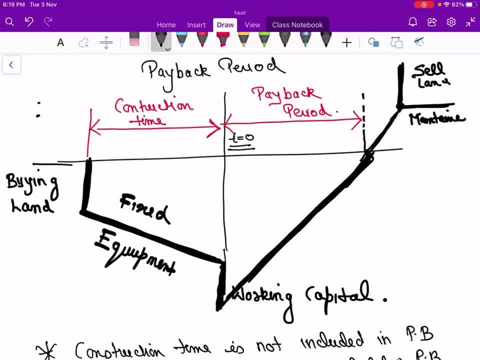 to include the construction time. Okay, So initially you have purchased The land. okay, initially you have purchased the land. after that you are going to purchase a fixed capital, that is, you are going to purchase the equipment and all that. okay, 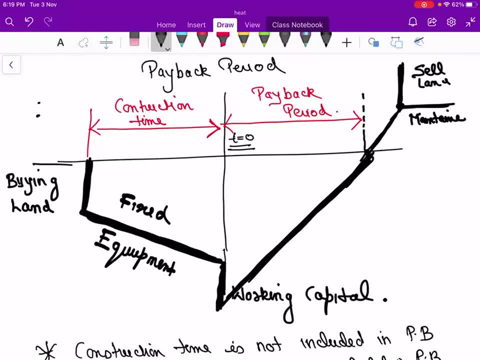 so this line will go slant. and once the plant is going to start, this is the point where time t equals to zero. once the plant is going to start, you need so much amount of raw materials. so this is the line again. drop in that due to the this. okay, this is the buying. 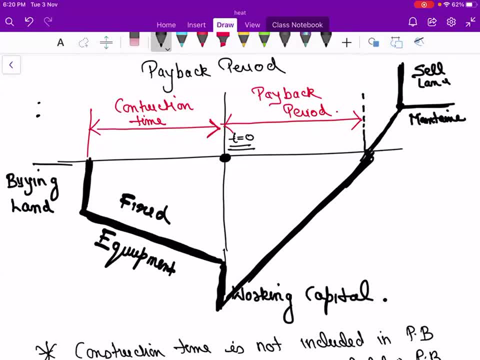 of raw material. you will need this. okay, so your plant will start here. Okay, Your plant will start here at bottom. okay, once the plant is started, okay, you will get a profit. you will earn a profit. okay, once it's going up, up, up, up and it will. 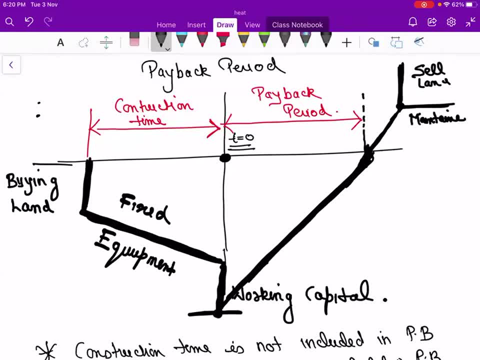 intersect the x-axis. okay, it will intersect the x-axis. so, basically, y-axis is for money- okay, y-axis is money and x-axis is time- okay, x-axis is time. so, once it intersects this, y-axis will intersect the. 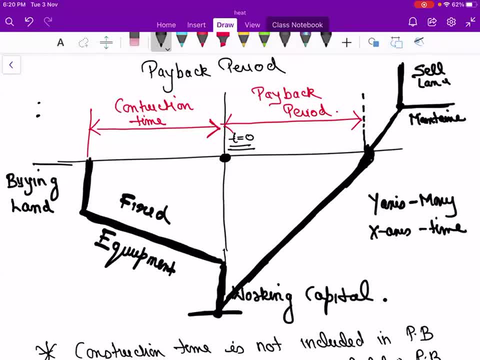 x-axis. here it is the time. this is known as payback period means your time will start from t equals to zero, when your plant will start. I have given example. okay, suppose the government decided today. okay, suppose the government decided today that they have. 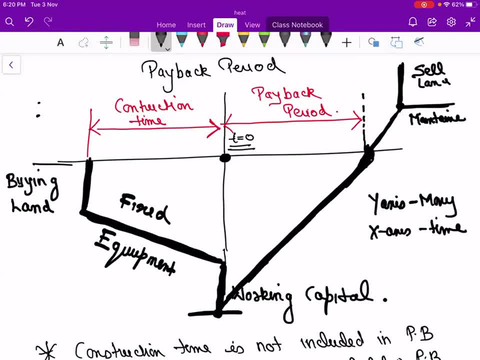 to construct a bridge? okay, they have to construct a bridge, okay. so the construction of bridge has taken, suppose three years, okay, after three years. suppose four years, okay. so after four years, what will happen? That road will start. 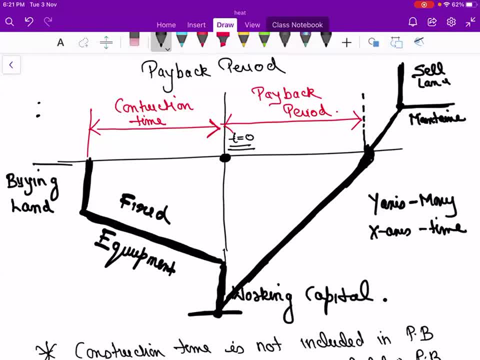 So you have to take the time when the road is started. okay, when the road is started, because from that day you will be collecting money. okay, from that day you will be starting or collecting money because the toll tax will start, So that is going to start. a collection of money will start from that time. 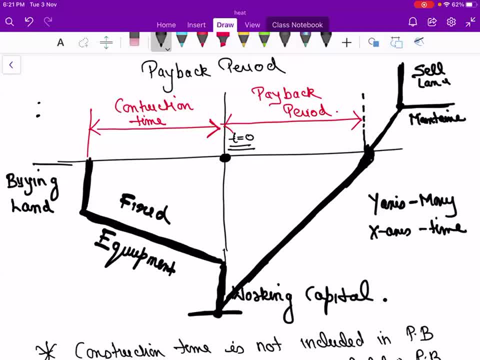 Okay, that is the time t equals to 0.. Okay, that moment your income is going to start. so that is time t equals to zero. you don't have to consider time t equals to zero from where construction is started. okay, you have to consider the time when your income is started from that source. okay, so that is time t equals to zero. 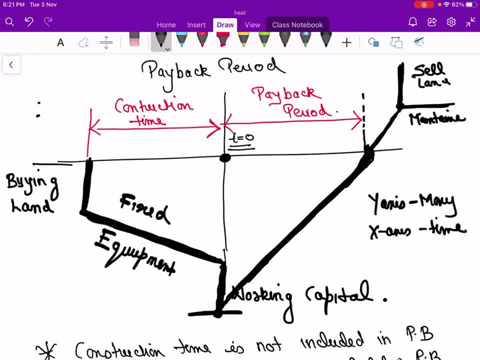 so it is going to recover your money. but payback period says you have to recover only your fixed capital equipment. okay, because working capital is it is a continuous term. okay, it is always, it will your, you will take always that money. okay means it will be requiring continuously that. 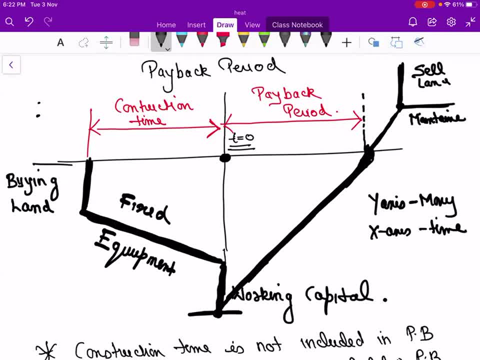 working capital. okay, and you will. you can recover the working capital at the end. okay, you can recover the working capital at the end, whatever the working capital you have. okay, so once you this intersect with the x axis and y axis, this time is known as okay. this. 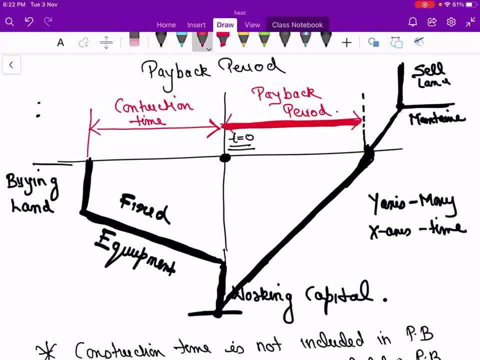 own red line is known as. this dark red line is known as payback period. okay, this red line is known as payback period, so with that the black line can go again up. okay, so you can sell land at that point, plus some raw material if you send. okay, so you can recover your some. 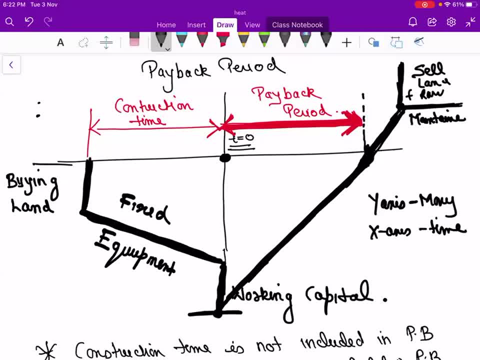 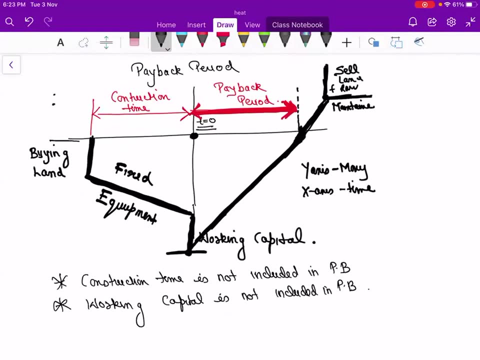 working capital also and that maintenance also okay. if it is going maintenance then it will be flat curve okay. so that's why i have given two points: strictly write that construction time is not included in payback period because we have to consider time when your plant is going to start. second, working capital is not included in the payback period. 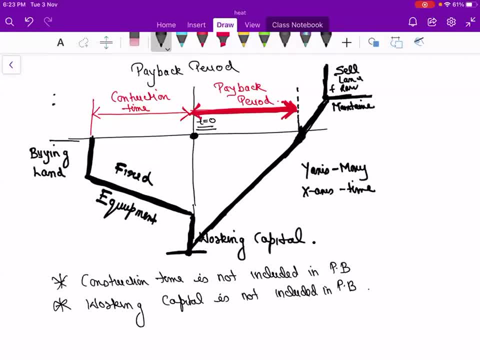 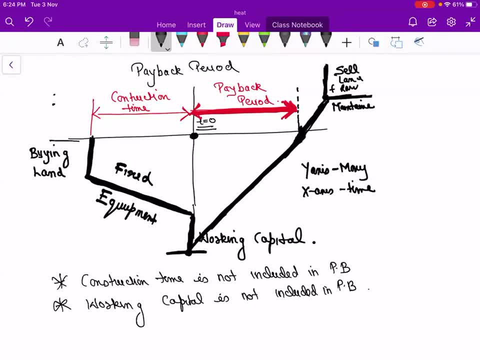 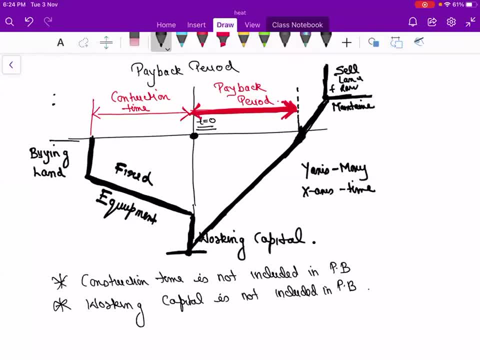 write that point. so, okay, everyone is saying yes, so write these points. i'm giving you two minutes, so thank you, venkatasai. okay, everyone got it. can we move forward? okay, fine, so what is if you someone ask you what is the payback period? payback period is the time in which we recover our fixed capital investment. 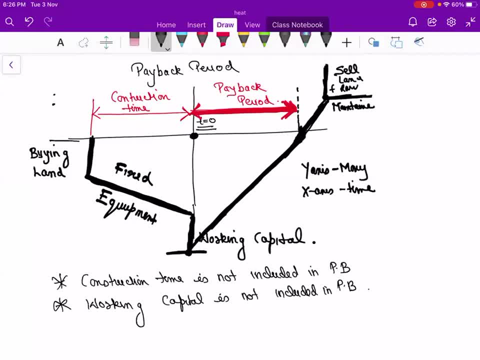 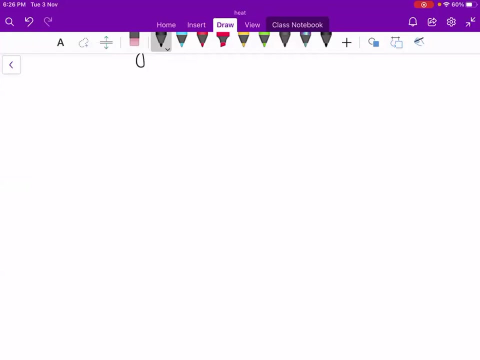 and in that we don't consider the construction time. okay, so this is the definition you have to remember. means: in payback period we consider only fixed capital investment, okay. okay, let's have a question. so to check whether you have actually understood or not the total fixed capital investment, 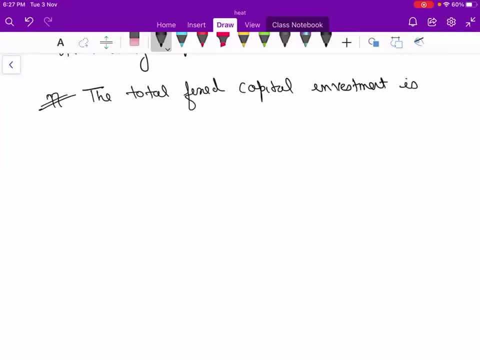 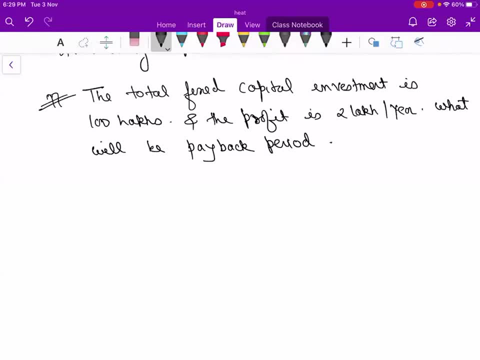 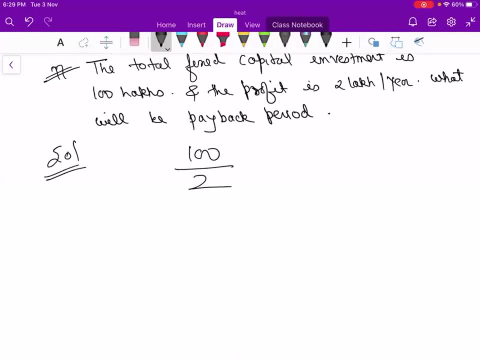 So the answer is directly solution: How much you have invested? 100 lakhs Per year. you are getting 2 lakhs, So answer will be 50.. 50 years, Okay. Next question: If the total capital investment is 80 lakhs and 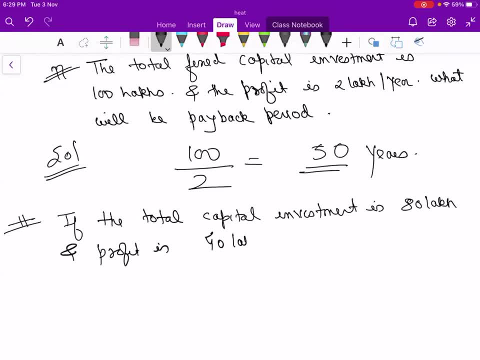 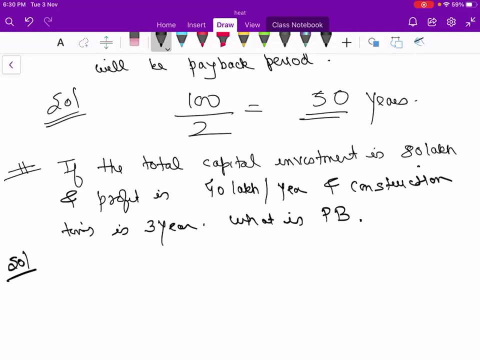 profit is 40 lakhs per year and construction time is 3 years. What is payback period? Okay, So this is a great question. Options are given: 2., 5., 3., 7.. This is a great question. Values may be different. Okay, But this is a great question. Solve it. 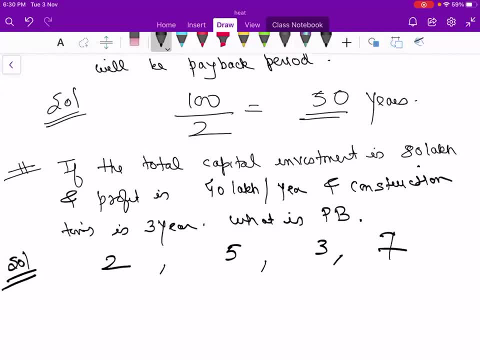 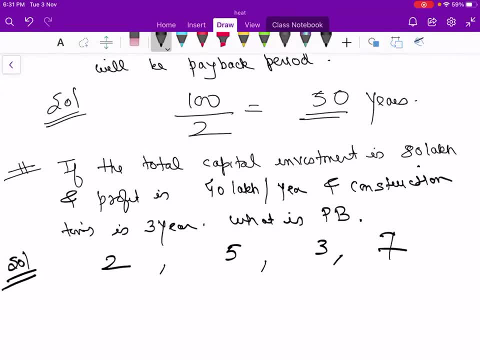 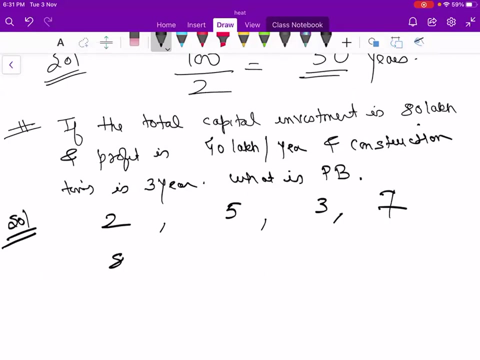 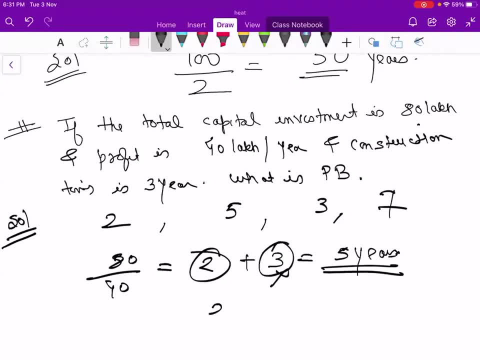 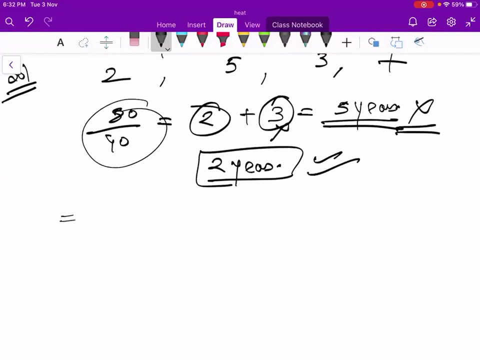 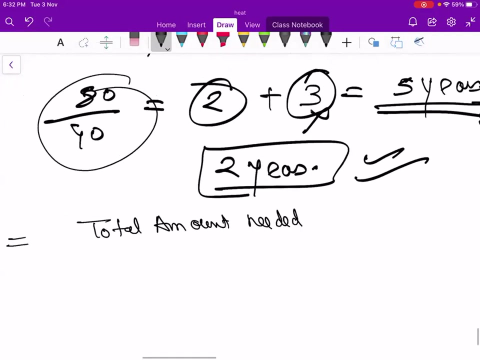 we don't consider this three, so the answer is two years. correct answer. okay, so this is wrong answer. don't do five years. okay, understood, everyone understood, yes or no? so what is formula here basically? formula is basically, if you see, that total amount needed, so it is basically fixed capital upon. 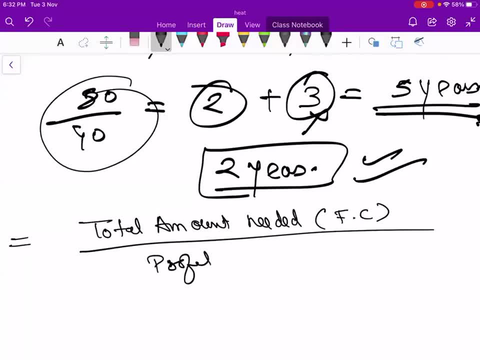 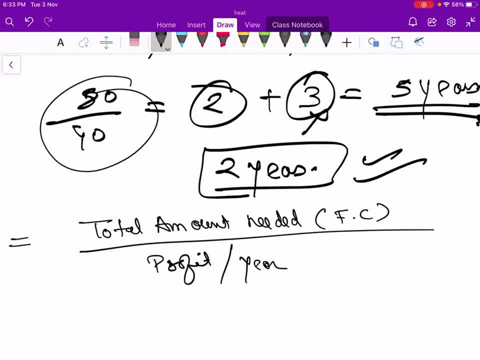 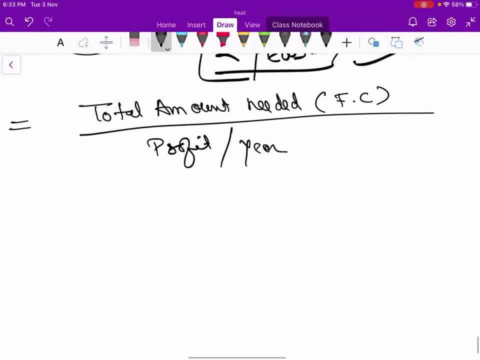 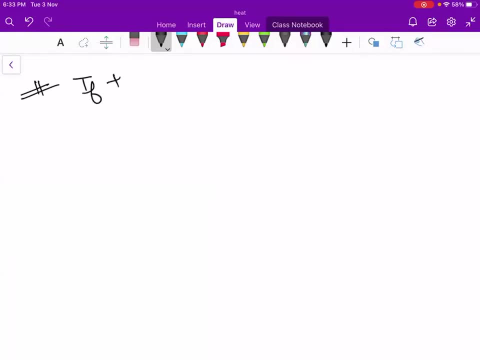 if the total investment is. so, if the total investment is 10 crore increased, the amount and profit is 2 crore per year, which makes this industry big. here calculate the payback. first, when money is not function, when money is not function of time. second, when money is function of time, I 12 hello per year. 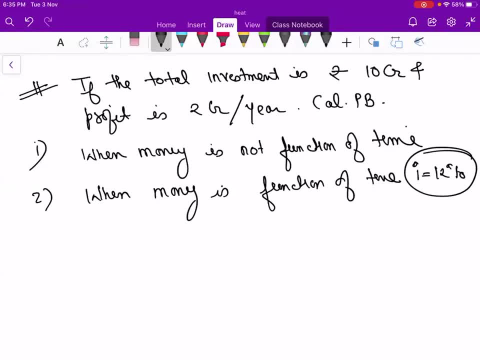 i equals you 12 year for 12 percent per year. now solve, okay, so money is a function of time. second, when money is not function, when I my time is not function of time, when some interest is there. okay, so that interest is 12%, it means it is. 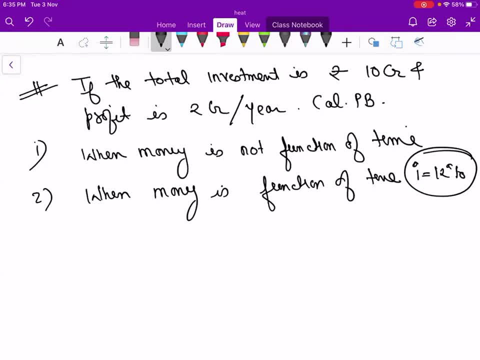 near to the mutual fund rate of interest. so we have seen that there are different rate of interest. that is first. one is the PSU's banks, like SBI, okay. second one: we have seen private banks. third, we have seen mutual funds. fourth one: we have seen share market, which is the very, very recent one. and then we have 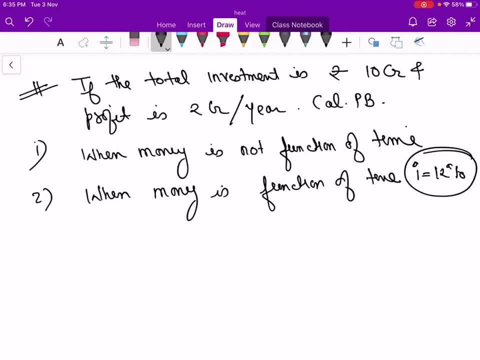 the masters as well. so this is a different you can see. so let's see what exactly everyone has most of it. so, basically, when you invest, when you are going to earn something, when you invest, try to bifurcate your money. okay, آمین, Come on. 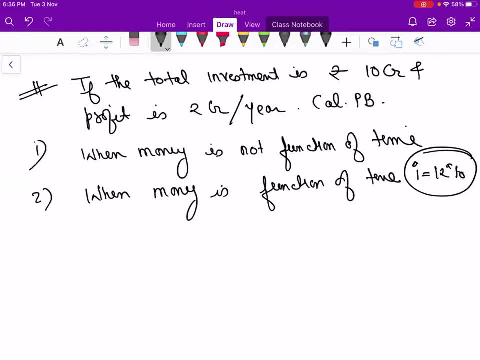 Aam absence: Syaam aam Blo. FEMA ingredie one section only. it's better that you buy for kit. solve the question, okay. I'm just saying solve it. I think this year the your semester exams will be late. almost everyone have a late semester examination. 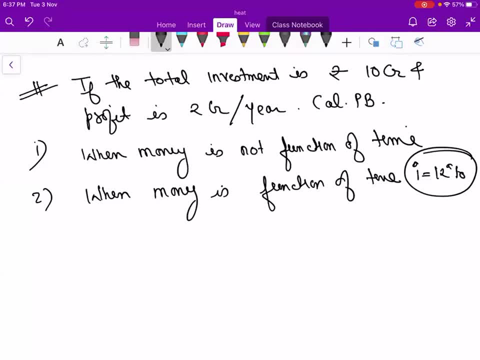 I think this year the your semester exams will be late. almost everyone have a late semester examination. all right, all right. service life- why you need service life here? there is no need of service life here. I think only one or two students got the correct answer. Solve it. I just attempt the question. 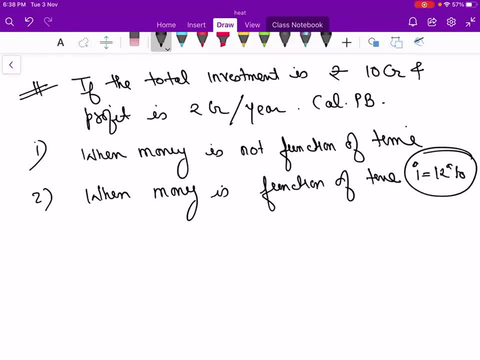 Solve the first. okay. Okay, Everyone got the first part correct. second part is: everyone is doing wrong, I don't know why. Okay, 67 students. Anjali, I think you got the answer correct. both answers are correct. 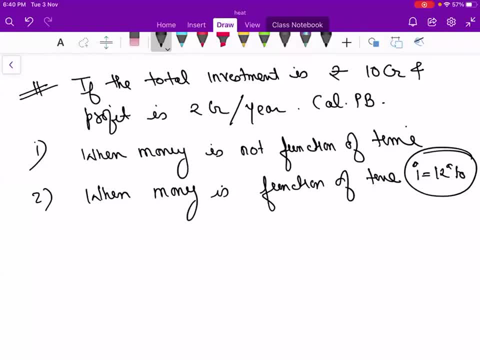 Okay, Okay, Let's solve the question. Okay, Thank you, Thank you, Great Thanks, Thank you, Thank you. Okay, let's solve the question. so first part, first part: 2 crore per year, 10 crore. i think this is the easiest question. 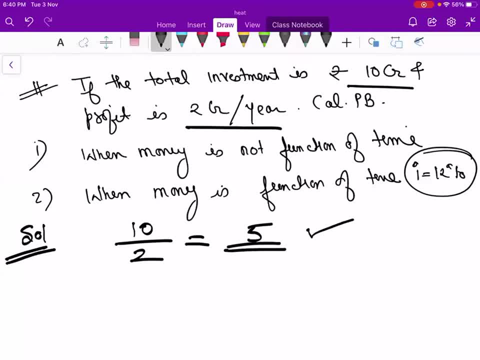 10 by 2 equals to 5.. i think in this no one has doubt. okay point is: when money is a function of time, okay, the total investments is 10 crore and the profit is 2 crore. once every year you are getting a 2 crore rupees. so when you get every year something, 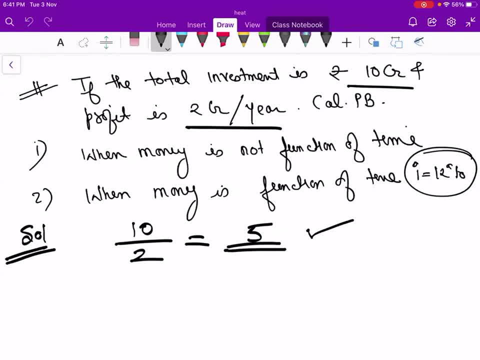 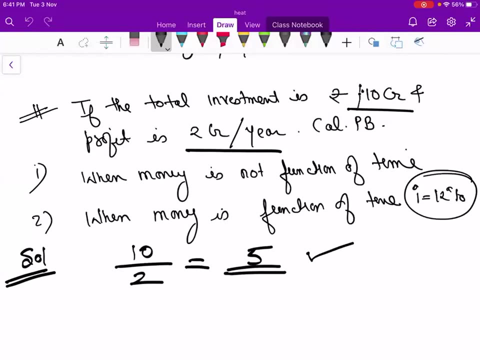 which formula we use when we get every year something? which formula we use? which formula we use annuity, very good, okay, very good, we use nvt. so what is the future amount here, or what is the present amount here? 10 crore, okay, 10 crore is the present amount. 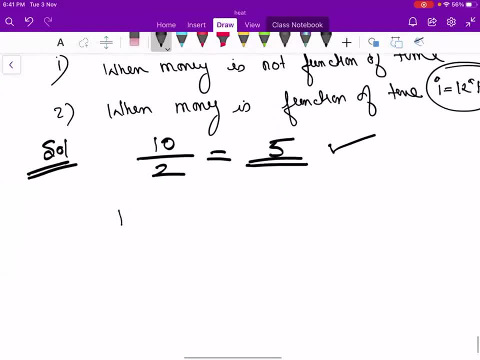 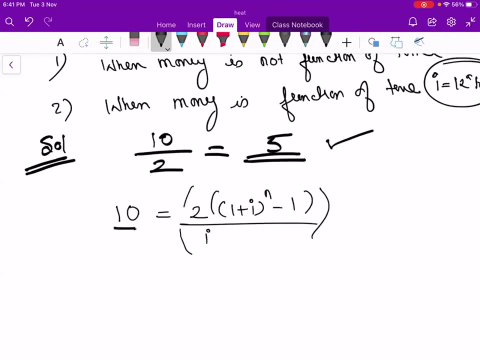 amount. okay, so formula will be: 10 equals to what will be the equal number of payments: 2. 1 plus i is given to the power n minus 1, okay, upon i, and this is present value. so this value also we want in present. okay, so divided by 1 plus i to the power n. 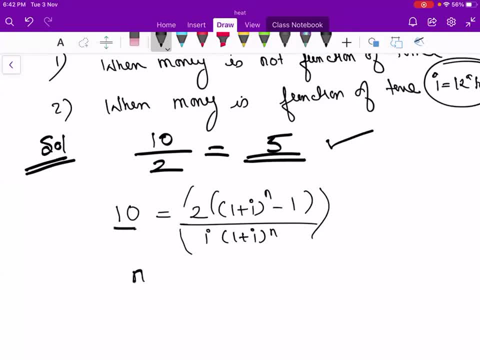 all this and i think your end will come eight years. yes, anura gopta, you have calculated correctly. say this: what is new in this? there is nothing new in this. you have to just think it: that every year you are getting something, when you get every or. 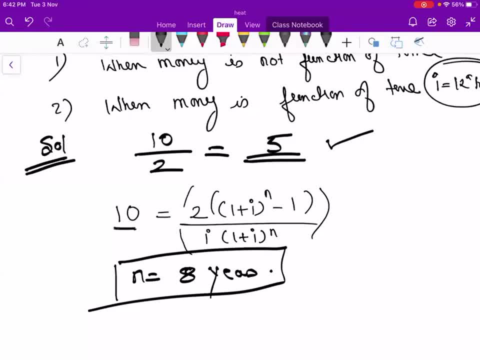 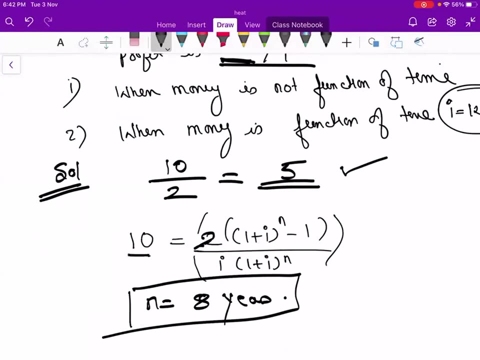 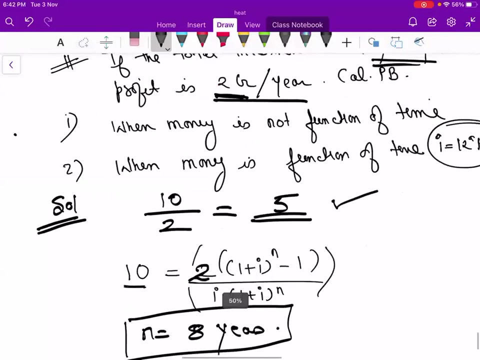 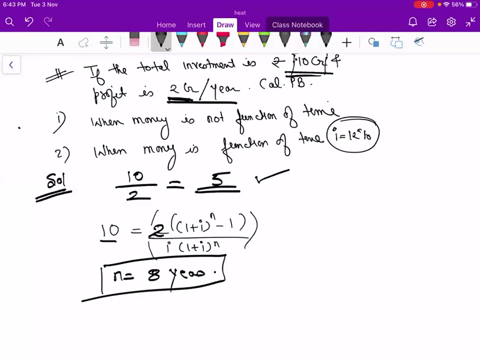 something it directly means. that means that you have to use a annuity formula. why 2? it is given in the question 2 crore per year. so that is why 2. okay, why interest only in 2 crore, not in 10 crore? okay, you want to take an interesting 10 crore also? 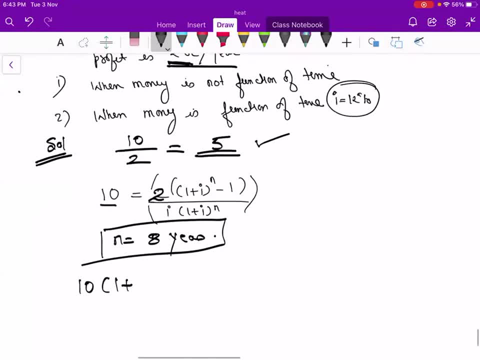 so write this equation like this: 10: 1 plus i to the power n equals to 2. 1 plus i to the power n minus 1 upon i. i have just taken this denominator term to this numerator. happy aditya demonstrators. hola samaj mariah kinney. IHR kina. yes or no? 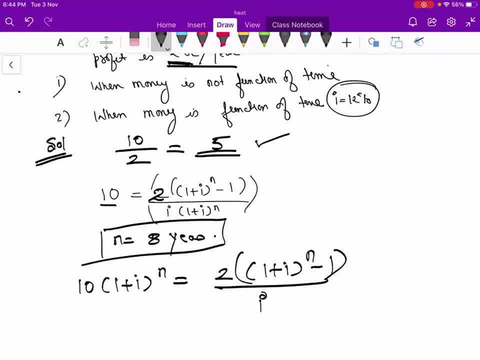 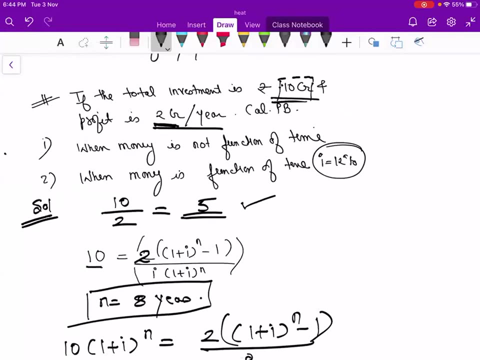 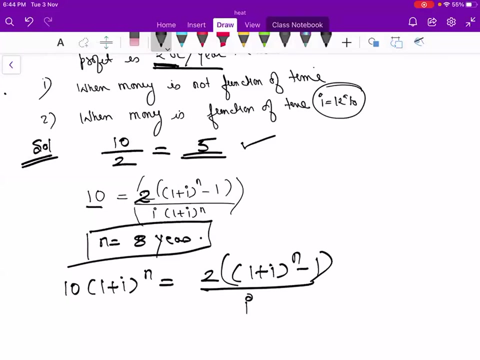 Did you understand or not? Yes or no? Why, too, it is given in the question 2 crore per year. Nachiket, when money is a function of time. your money increases or decreases. Nachiket, when your money is a function of time: it increases or decreases. 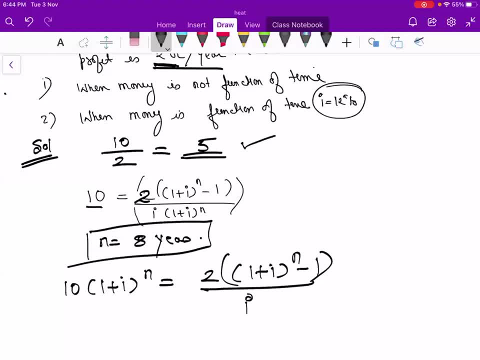 Increases. So that's the answer: 21176, how it decreases. It means that when you put money- rule number 21176,, when you will put money in the bank, your money will decrease. Okay, it will always increase. 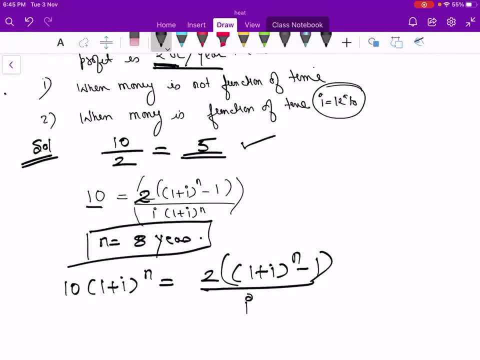 Okay, fine, So anyone has doubt. Everyone is now comfortable. Profit how profit will increase. It is clearly mentioned in the question It is 2 crore per year. Why you are assuming unnecessarily data. It is clearly mentioned that it is 2 crore per year. 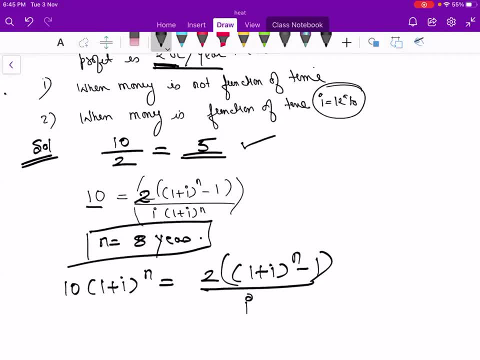 So how profit is going to increase? That value may increase, but the number 2, crore, is there, Okay. So tell me, did you understand or not? Everyone just reply. Everyone reply yes or no. It is failed. Everyone reply yes or no. 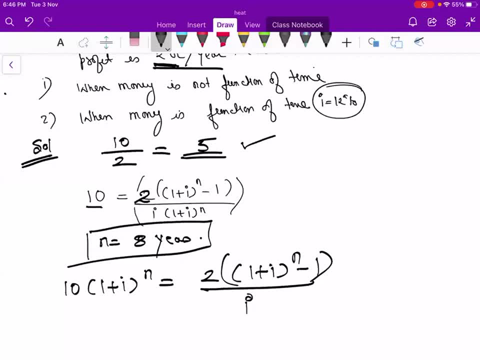 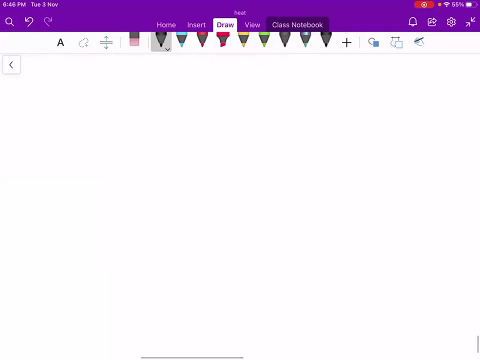 Everyone reply yes or no. Everybody reply yes or no. Everyone is comfortable. okay, fine, we will go to the next question. a polymer plant with production capacity of 10,000 ton per year has an overall yield of 70% on mass basis, kg product upon kg raw material. 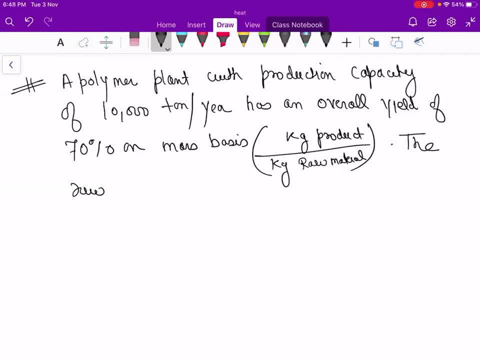 the raw material cost. the raw material cost is rupees 50,000 per ton. the process modification is proposed to increase the overall yield to 75% with an investment of 12.5 crores. i equals to 12 percent. calculate the payback period. 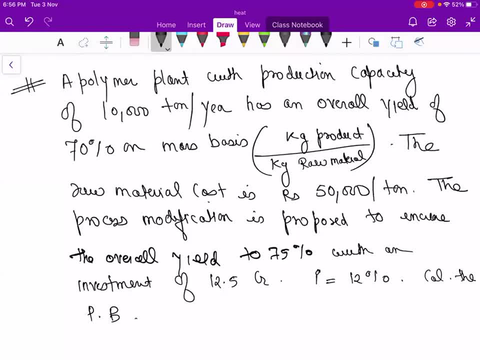 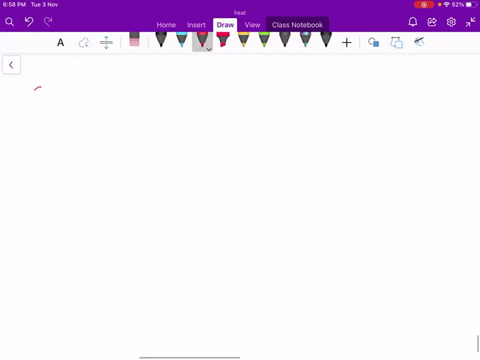 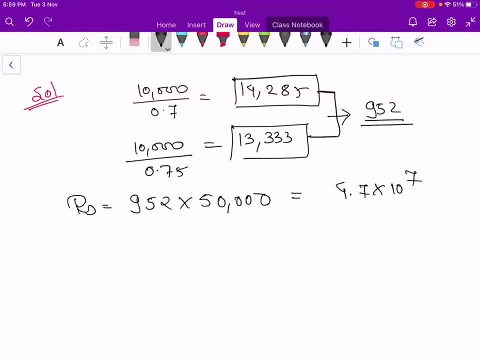 3, 3,, 4,, 5,, 6, 7.. Okay, 4.76 crore. Okay, This is the thing you are getting. So what will be the payback period? just payback period. how much you have invested, 12.5 into? okay, 12.5 into, uh, how much? 10 to the. 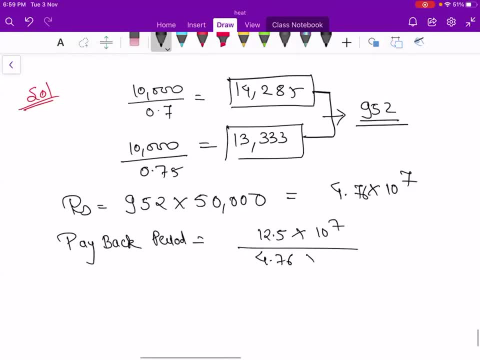 power 7 and it is 4.76 into 10 to the power 7. so what it is coming, i think it will be 4 to the 8 2 point. something will come okay. 2.62. yes, so this is the payback period. 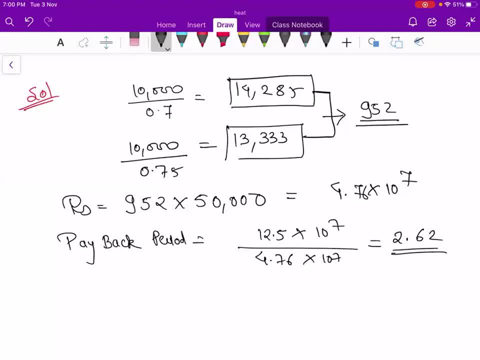 okay, so 952 kg of raw material you are going to save and you can calculate from this that this much amount of money you are going to save every year. okay, so, this much amount you have invested. okay, this much amount you have invested, so this is the payback period. 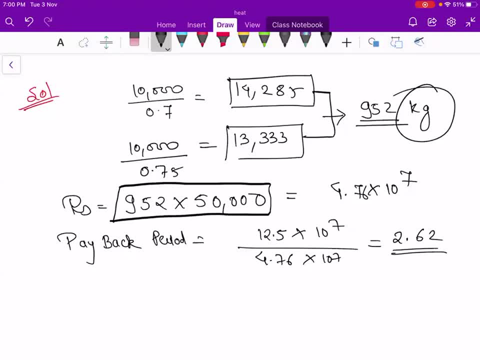 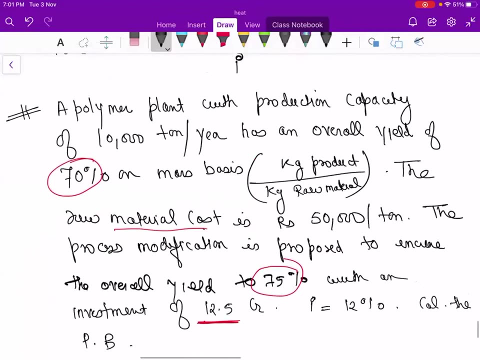 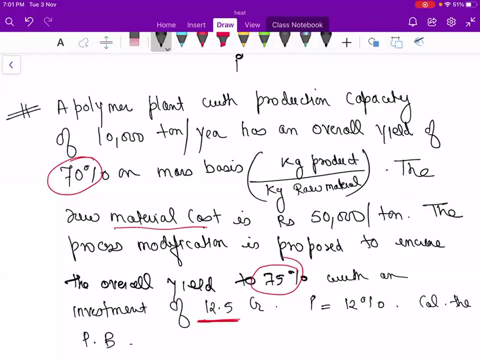 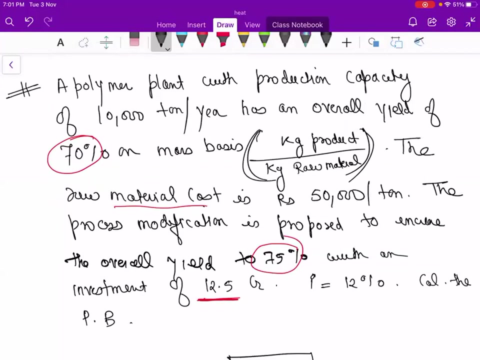 see, it is given that a polymer plant with production capacity of 10 000 ton per year has an overall yield of 70 percent on mass basis. okay, they have given on mass basis. so the raw cost is 50 000 per ton the production. the process modification is proposed to increase the overall. 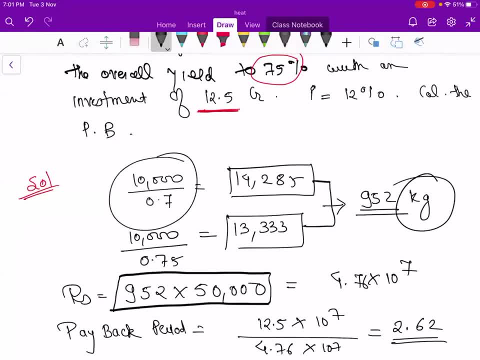 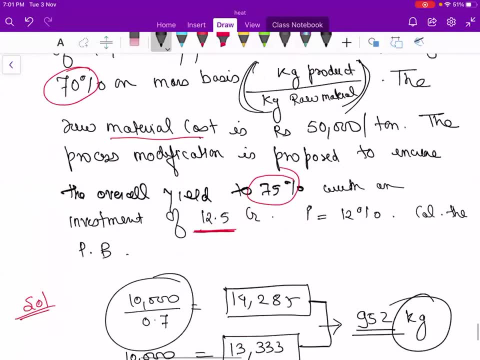 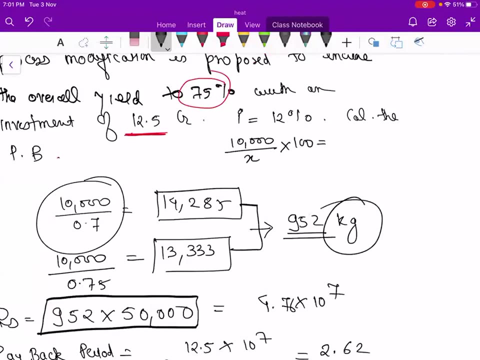 yield to 75 percent. so just, i have written nothing, it is the formula. okay, i have just written a formula for this, so it is. they have given itself the formula kg of product upon kg of raw material. so it is 10 000 divided by x into 100. so this year i have given 70 percent, okay. 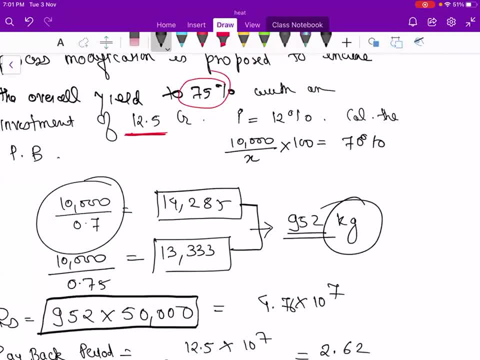 so biggest problem is that give the plus or minusth rate ofmind- i hide it- to the 10 집, small withdraw, i will put something big order called 5500 and money will be 952. so this for 9Box. after this we will solve. or we will solve for when money is a function of time. after that we will solve and money is a function time. so for here you will get 952, okay, so 952 x to 50 000 will be 952, 0 with 8 money and you get 953 x to 10 pockets. so this is what you have, Definitely segment, okay. so first we solve when money is not a function of time, okay, and if 대통령, than we will solve when money is a function of time. so for here you will get 952, okay, so 952 x to thank god also when money is the function of time. so here, x, you will get 952, okay, so 952 x to thank god also. 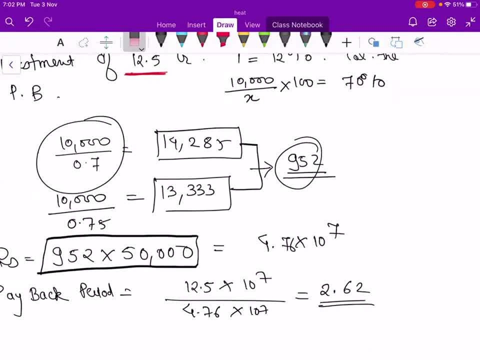 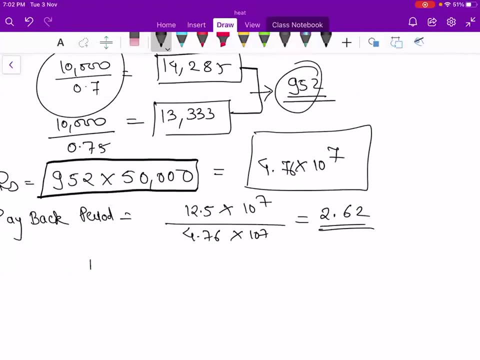 So 952 into 50,000,. okay, so this much amount of money we are going to save every year. Okay, So this. so if, when money is a function of time, you can just solve it like this: 12.5 equals to how much it will be four point seven, six, one plus I. value is given to the power n minus one. 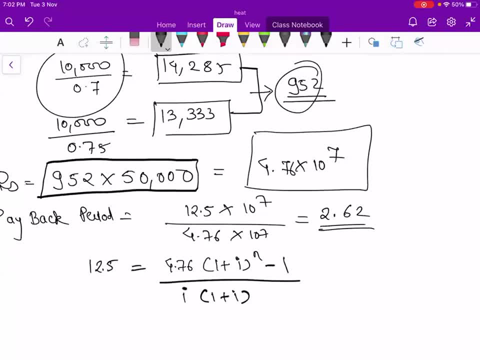 upon I One plus I to the power n. So from here also, you can calculate, then, and this n is a when money is a function of time. Okay, here, money is not a function of time. Okay, Yeah, you can not cross. Okay, money is Not a function of time. 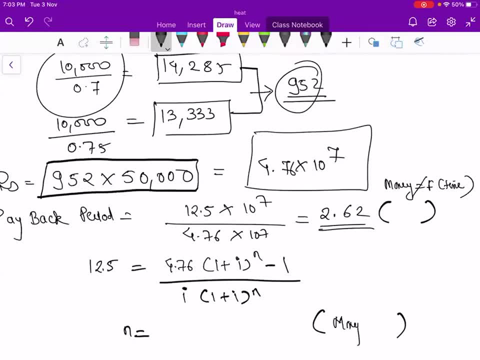 Here n is: money is a function of time. So How much answer you are getting when money is a function of time? How much answer you are getting when money is a function of time? 3.4 years, okay, Okay, so this is the answer. everyone, what this? 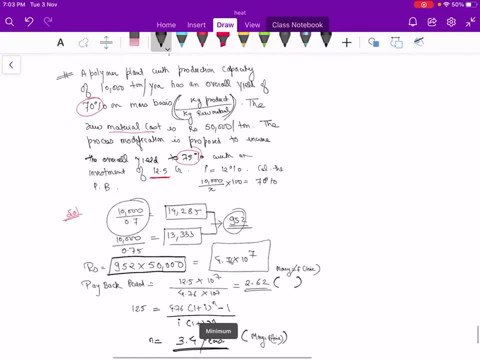 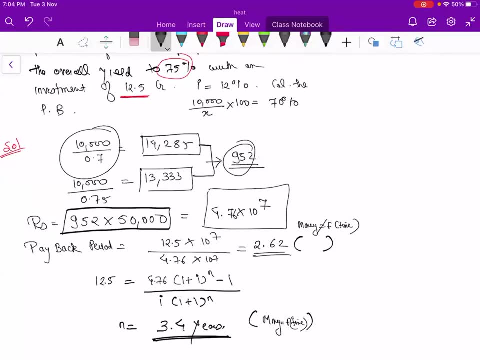 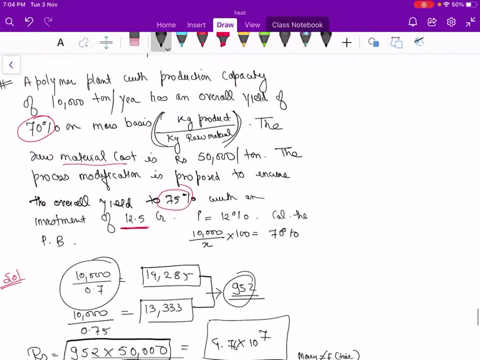 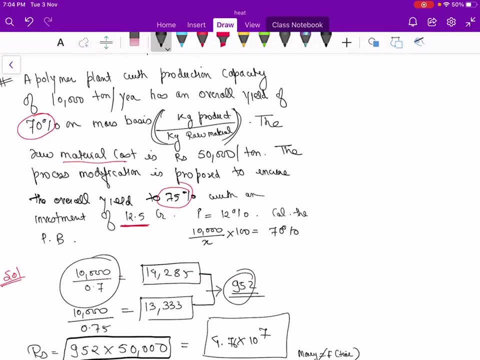 You can see now You can see in a solution. Just read the portion again. okay, some students have doubt, so they did and again solve it. Okay, I'm given two minutes. read it and try to see what they have asked and what you have to calculate. 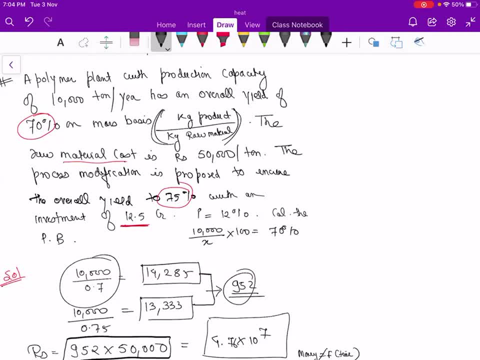 Okay, Basically here. see, they have not mentioned basically whether it is a working capital or this fixed cost. okay, just they have given. you can't say that here this is a working capital. So how can you solve this question? 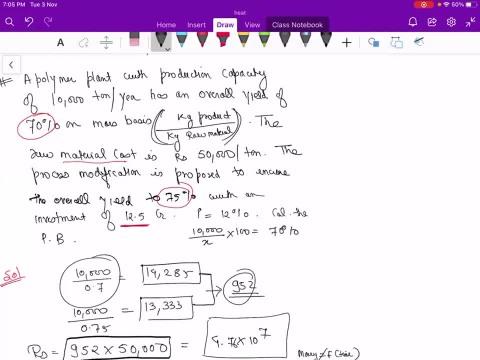 This is a great question, Okay, So basically, some amount is they have deposited, so you will be saving some money in that. this is a payback period, Okay, in this question, but exact definition what I have told that you have to remember. 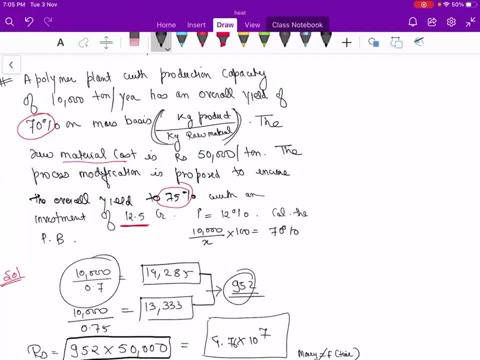 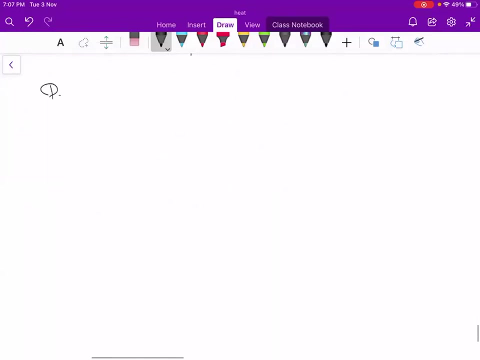 okay, So everyone is clear now. Okay, So everyone is clear: yes or no, Yes or no, right, Okay, fine, Yes or no right, One is the only one. Yes or no, Yes, Yes. There is one formula for payback period also, that depreciable fixed cost. okay, so if in 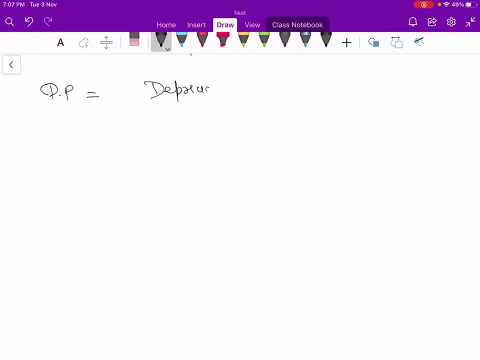 the question. it is given depreciable fixed cost, so in the denominator you have to add it: per year plus depreciation. okay, so this is the formula for payback period. okay, if depreciated amount is given, so you have to add that depreciation in that. okay, so this: 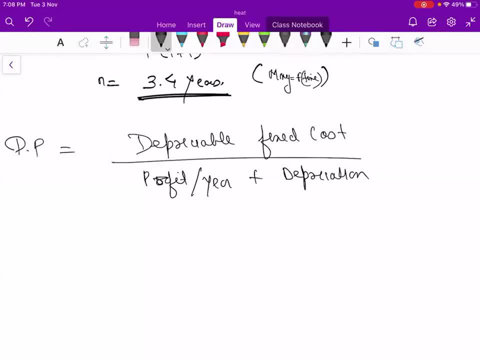 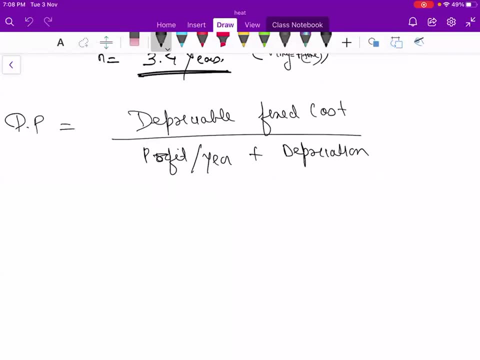 is the question which get has asked one time. okay, so in that the question is like this: the depreciable fixed cost is rupees hundred lakhs and the fixed cost is rupees hundred lakhs and the depreciable depreciable, depreciable. 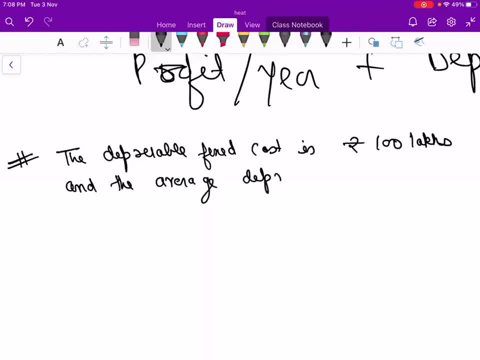 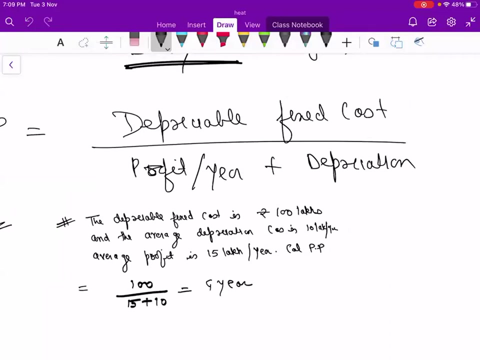 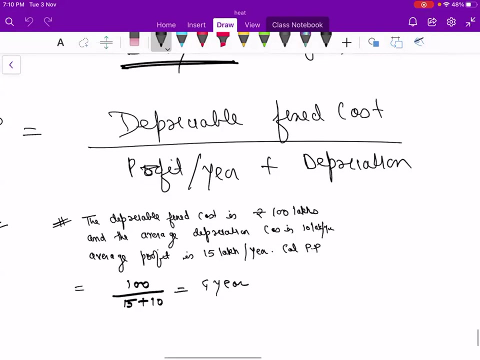 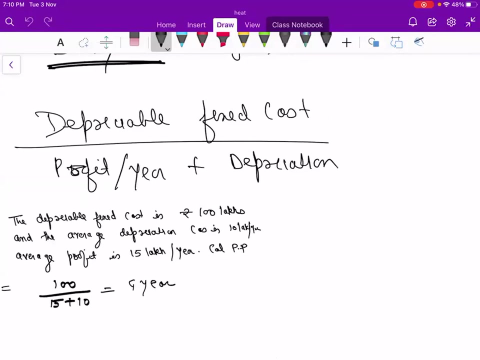 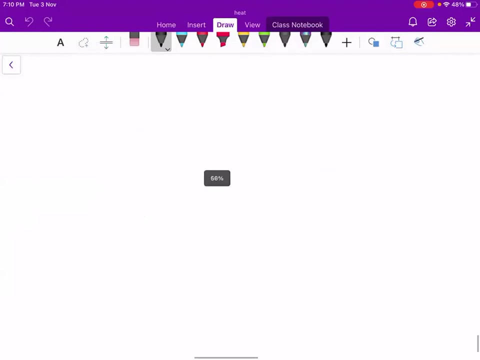 depreciable, depreciable depreciation cost. is that the, that, the that that that payback period? so calculate it. yeah, correct, so it will be hundred plus 15 plus 10 equals to four year. see the formula. everyone got this answer. yes, socket, okay. so next question we will do now, due to twenty percent, due to twenty. 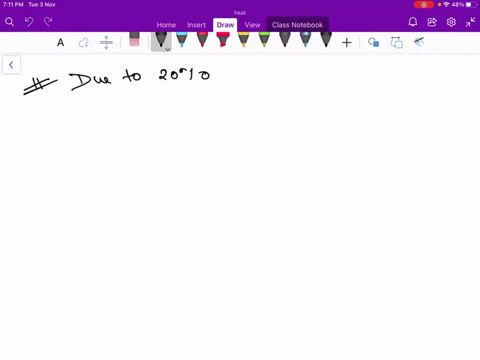 percent, 20 percent, 20 percent, yes, yes, yes, yes. drop in the product. due to 20 percent drop in the product selling price. the payback period of new plant is increased to is increased to 1.5 times of estimated initially. The production cost, CP and production rate is constant. 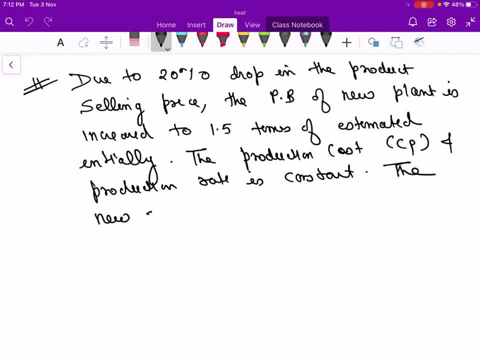 The new selling price is CS. The new selling price is CS. The new selling price is CS. Calculate the ratio of CP by CS: okay. Calculate the ratio of CP by CS: okay. Calculate the ratio of CP by CS: okay. 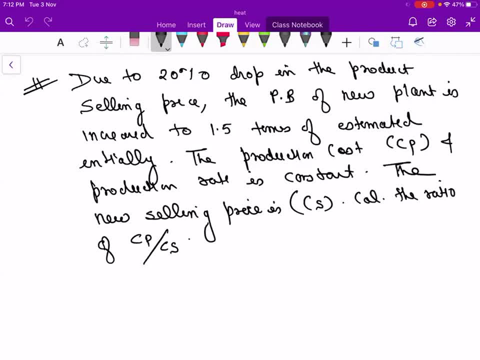 But in the question, if we take no, you can't take socket, that 100 because in numerator it is depreciable, cost is given okay, So you have to add in the denominator. So you have to add in the denominator. 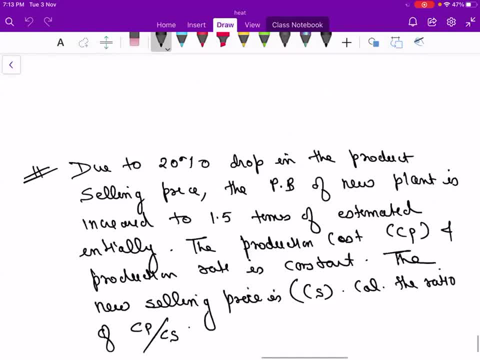 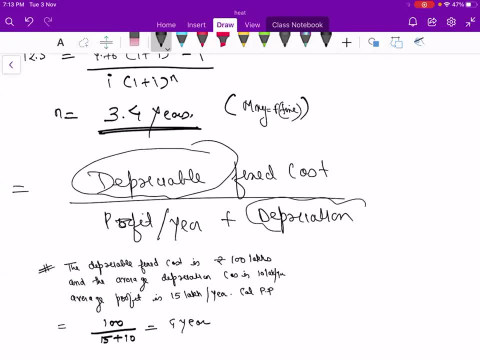 I don't understand how the formula came. It is just in the previous formula. If you are adding depreciable amount, okay, In the numerator, so you have to add that into denominator also, Okay, Just remember this point, Okay. 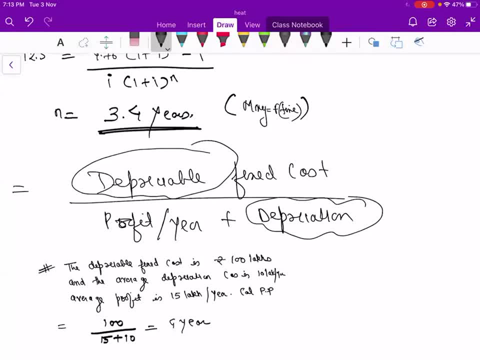 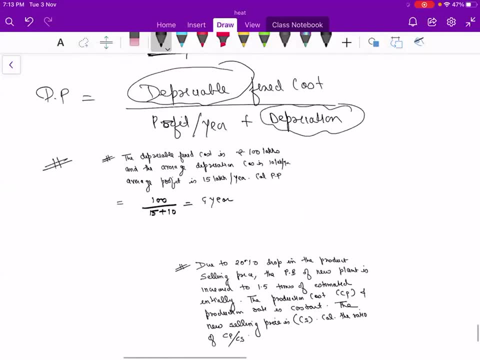 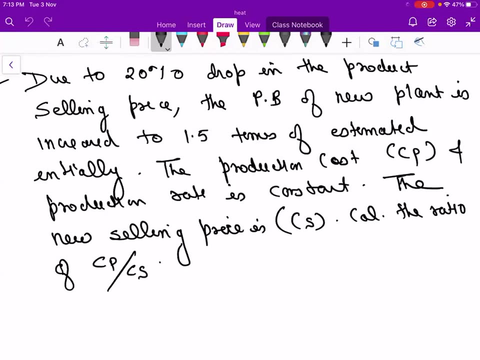 If something is numerator, then that should be in the denominator. That's it, So that's it. That's it, That's it. Solve this. This is a very good, great question, So please solve this on your own, Okay. 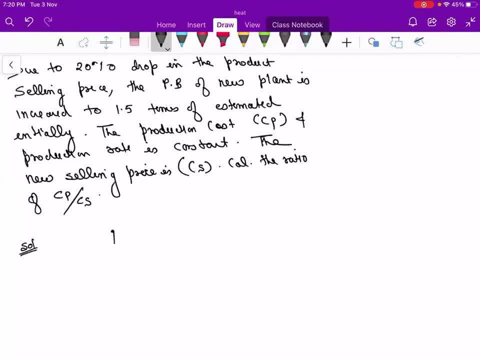 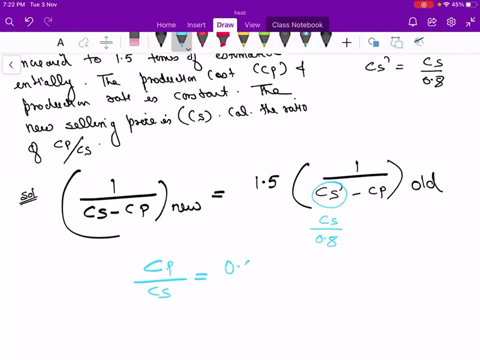 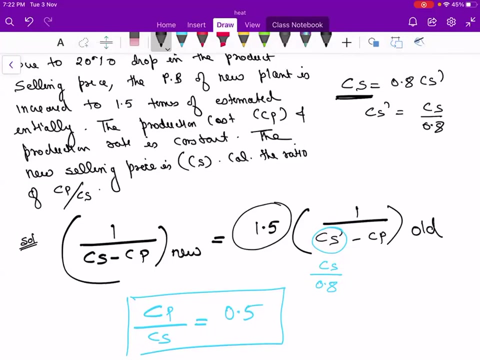 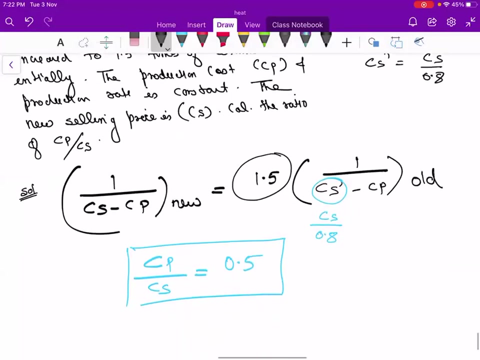 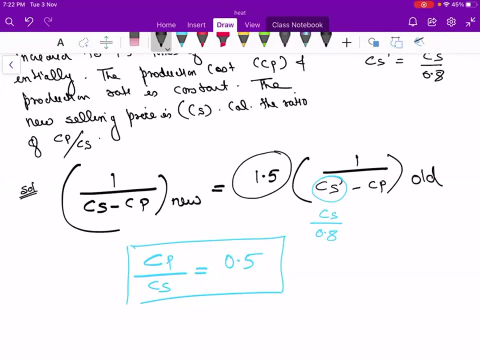 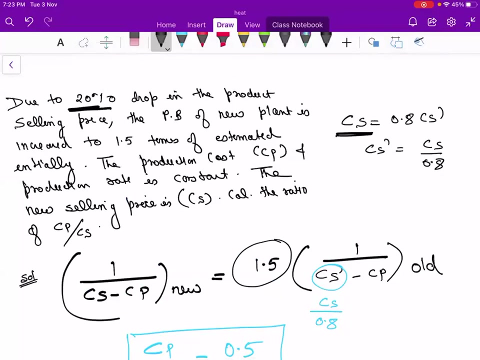 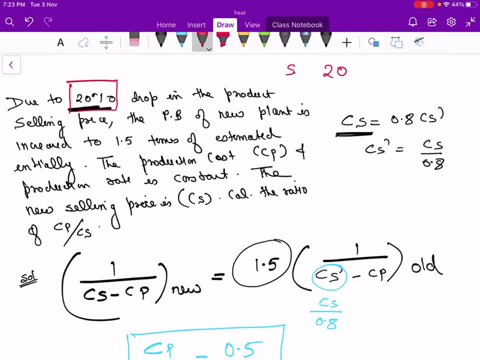 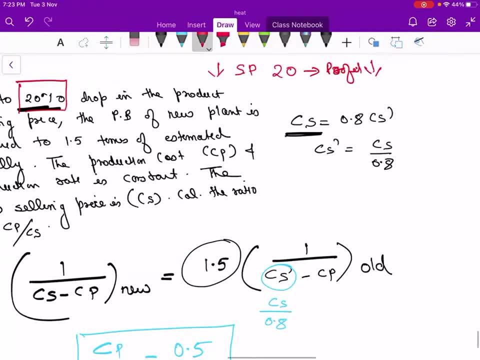 so selling price is going to drop, what does? it means your profit is going to drop, okay. if your selling price is going to drop, your profit is going to drop. it means payback period will going to increase. okay, because it is in denominator, profit is going to increase, okay. so if you are, selling price is going to 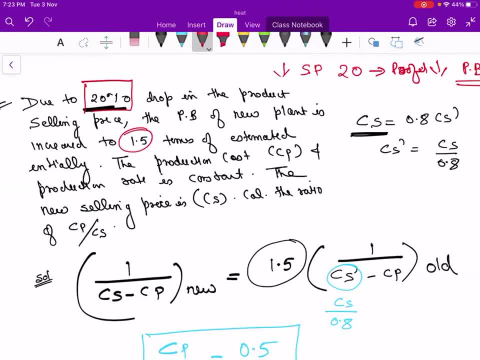 drop value as a new profit term. okay, so they have given, it is 1.5 times. so they have given means new is 1.5 times. it has increased to the odego, an suggest we have taken. so in numerator it is, in numerator it is investment, so you can. 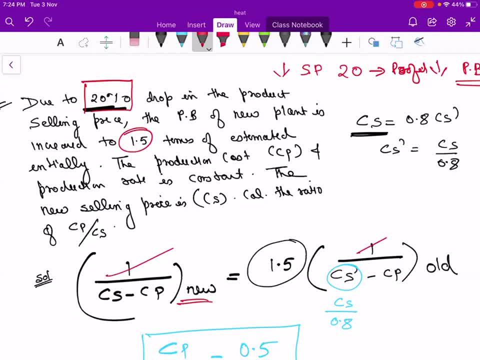 take it 1, 2, 3, any value you can take. so this will just cancel out, okay你, because investment is same. see, it is given the production cost, CP and the production rate is constant and everything is faith here. only changes just it. so we have calculated this, so old CS they have not given. so that is. 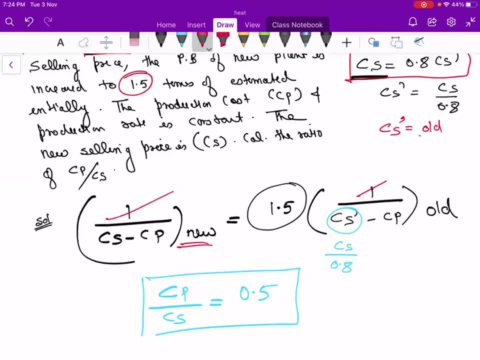 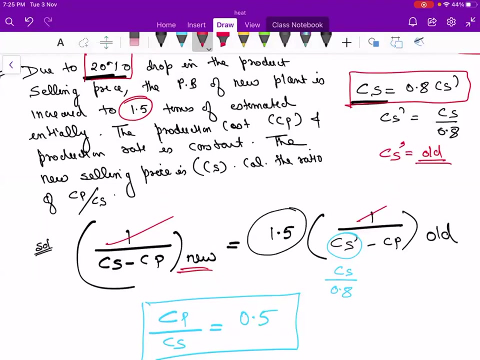 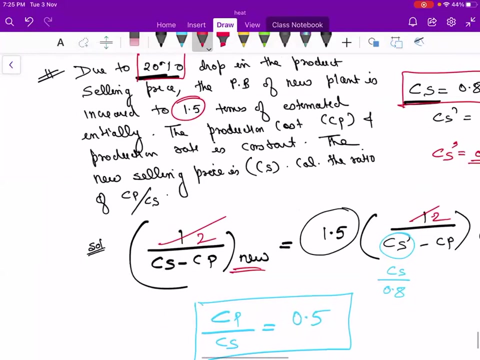 why this is CS that is old, okay, so that is why we have taken here. I haven't got this point, yeah, so I have written this now: 0.8 CS CS, new CS is reduced now how CS dash is reduced and Raghuta: 2: 1. 1, 3, 8, 2. so why I have taken: 1 here, you can take it. 2 here, 3 here, any value. 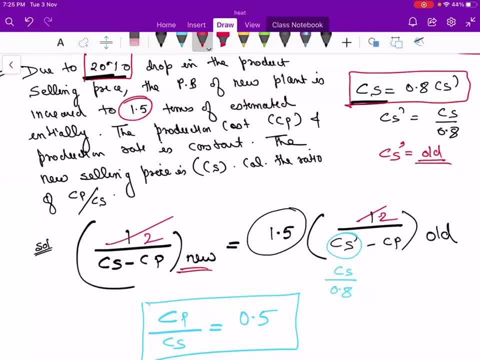 you can take. now, this is the investment, so investment is same that is given in the question. so that is our base value. I have taken 1. you can take it. any value that will be cancelled it out either. you can take it. CP means how much one is. 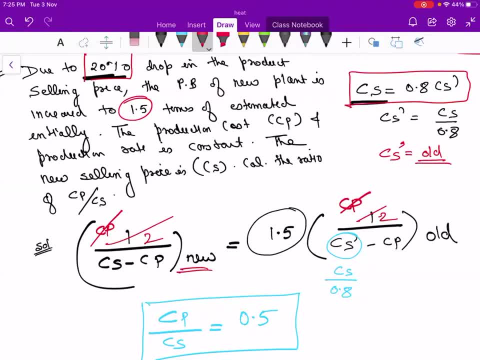 required for the production. again, that CP will be cancelled because that value will be same. okay, 2, 1, 1, 3, 8, 2. yeah, you take it. X, Y, Z, any value, okay, it doesn't matter. okay, that is same, that is important. okay, I have not taken X because 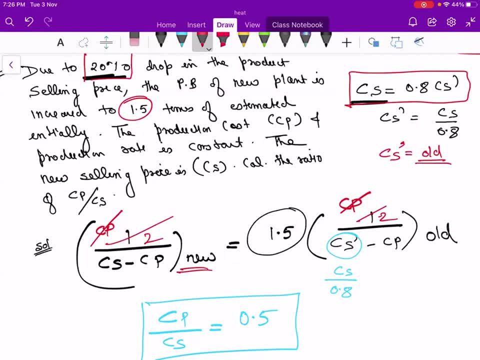 if I take X, then most of the mind will think that we have to calculate X. okay, so we don't have to calculate X there. see it's on you. you take it X, you take it 1. Okay, you take it. gamma, alpha. you are it? go 1 over some. 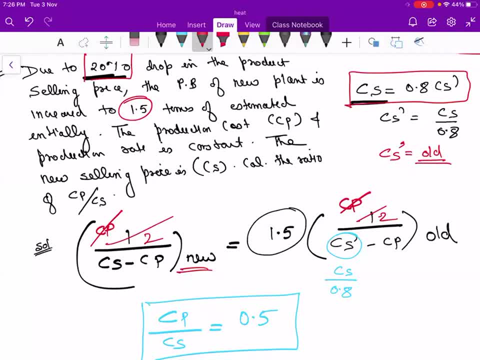 님, yeah, no problem. so say you take it 1 or get leap 1 or 2, 3 is the EASIESTẽ1 all 2, or take it 2 or take it alpha. you are not stable to solve this question. why- and this is one of the easiest subject- you are in third years or final year? two, one, one, three, eight, two, radiation person factor or final year, three, two, Third Year. okay, so this is easy. subject when there is nothing in the role is easy. subject in the role is easy, readily okay, so this is the one of the easiest subject. one there is nothing in the role is easily. declaration of any student's. 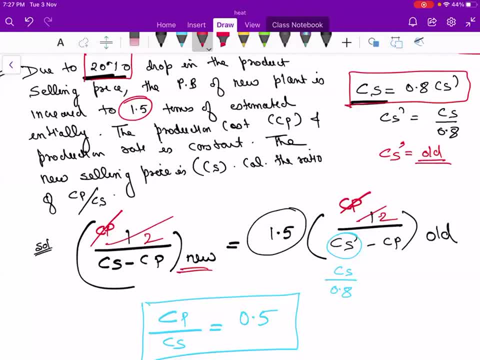 but in the point that some don't find it difficult, but in the point that the point to some student find it difficult, does it mean that work hard technology or is there? there is nothing thing like that. just the point is that some students find it difficult because it is economics. okay. 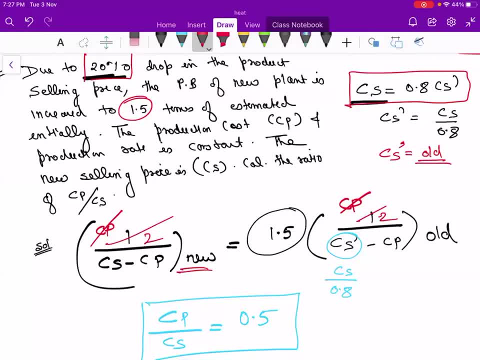 it is not a chemical engineer, a technical subject. okay, so there are some new terminologies are introduced here. okay, so you should be familiar with this and I think we are going with a very medium pace. okay, I am NOT going too much slow, I am NOT going too much high speed. okay, except 2: 1, 1, 3, 8, 2 other students: 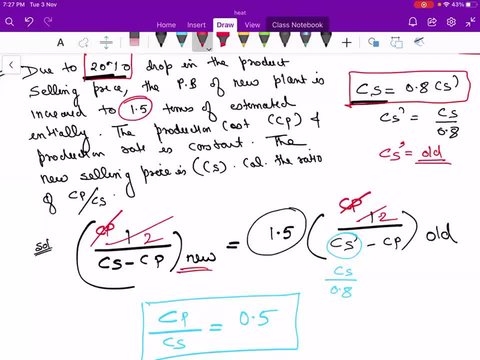 anyone has problem, then I will think on that. if you are getting all the points or not, other than roll number 2. 1, 1, 3, 8, 2. anyone has problem? everyone is comfortable, yes or no? please reply? please reply other student. yeah, cannot solve every question immediately. it depends on how much you. 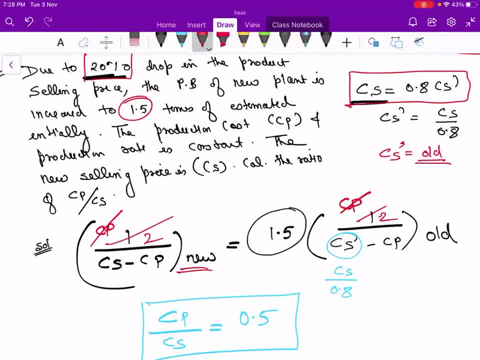 do practice okay, so don't worry about that. the point is: you are getting the concept or not. okay, after revision, you can easily solve the question. okay, please reply. optimum topic. you have problem? see, optimum, actually there is no formula. okay, optimization: there is no formula. that is the only topic where you don't. 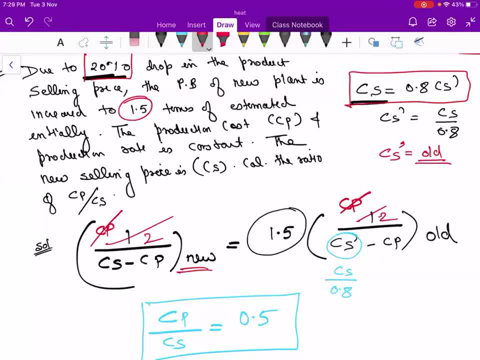 have to use any formula, just differentiate it. okay, If you have a problem in making equations, then you have to read the portion and see that what data you can extract from there. This formula we have just used, the formula of total investment upon profit. This is the formula we have used. 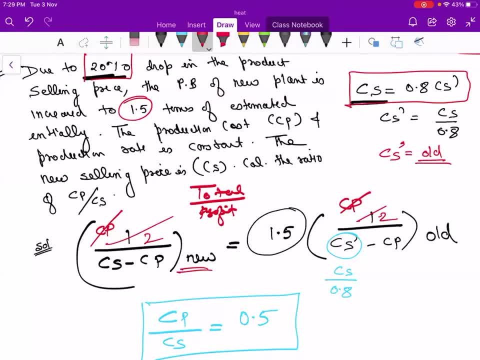 So CS minus CP will give you profit and your total investment is same in both the cases. Any other feedback? Yes, I cut just one saying that you are not today. I thought you are not giving answer today Every time you sleep. okay, in that is that I'm teaching boring, or this is your sleep. 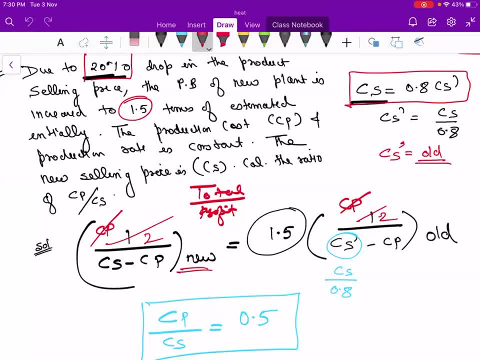 time. Others reply: Everyone is comfortable. Okay, fine, So there are still so many questions. Okay, So before that, I will, I think I will teach a theory so that we will be able to do it. Okay, Okay, Okay. 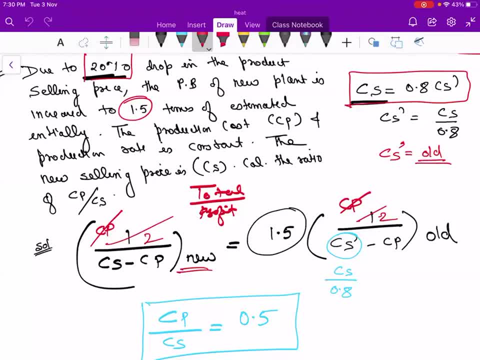 Okay, Okay, Okay. Okay. Now I will complete with that theory today, And some questions are there that we can do afterwards. So tomorrow we will do the pump. So tomorrow, two and half up to three hours, we will be doing pump. 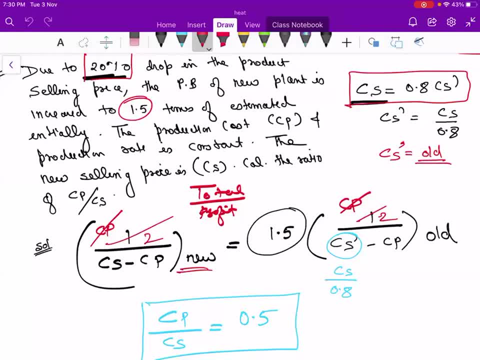 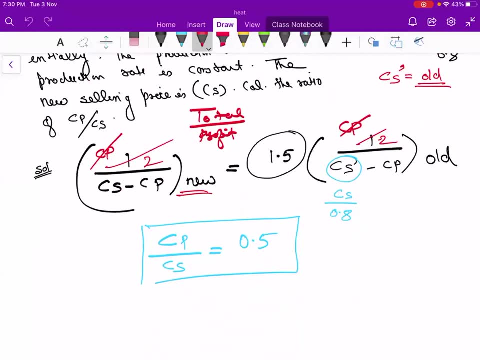 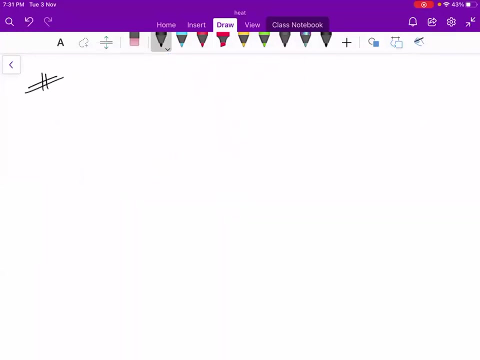 Okay, So at least theory part we will complete today and some practice questions we will do at the end of the sessions. Okay, Okay, are remaining okay, so see topic. rate of return: okay, so rate of return means basically profit and total capital investment profit annual. so by default. 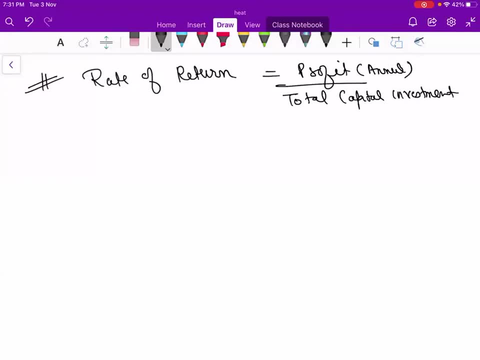 we take profit without paying the income tax. okay, by default, we take the profit without paying the income tax. if it is mentioned in the question, then you have to subtract the okay. if you have to mention, if it is mentioned in the question that profit income tax is this much, then you have to subtract it. okay. 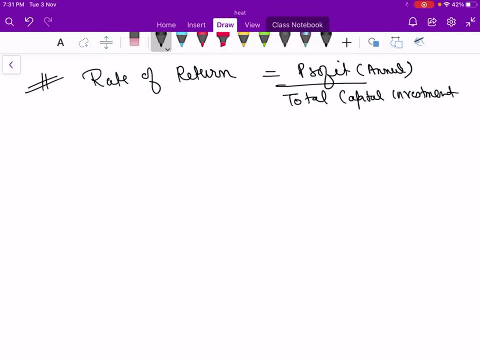 so, by default, the formula for rate of return is profit upon total capital investment. okay, okay. so one question: the total. you? you invest, investment, investment, investment, And the total investment in a project is rupees 10 lakh and annual profit is rupees 1.5 lakh. 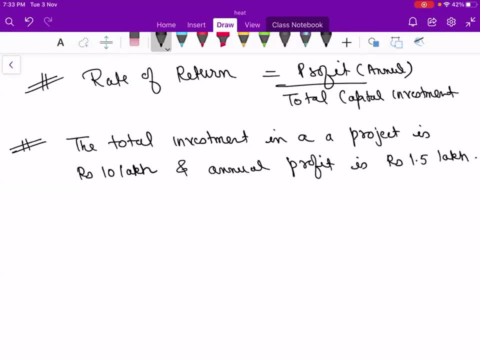 Okay, And n equals to 10 years. Calculate rate of return: ROR: Yes, 210524, you can say. but exactly, you can't say Okay, there are various terms. Okay, Okay, Because in that you have to consider the rate of return. 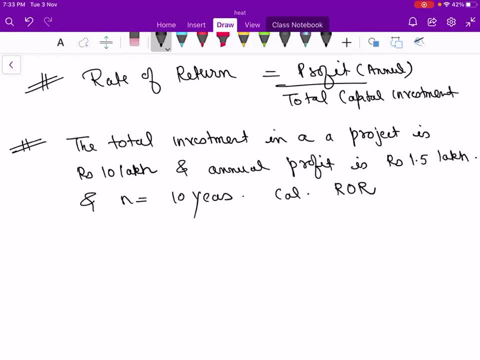 You have to consider only fixed capital. Okay, Yes, correct. What is your name? Venkata Sai? Yes, your answer is correct. Yes, we will do discounted cash flow. Okay, Okay, Okay, Okay, Okay, Okay. 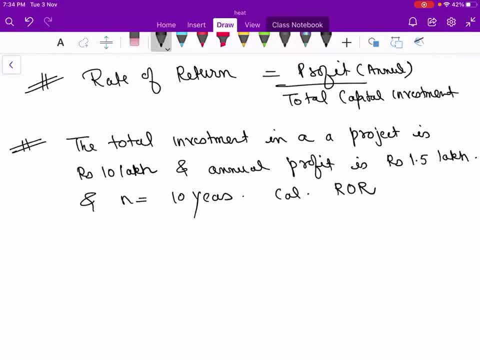 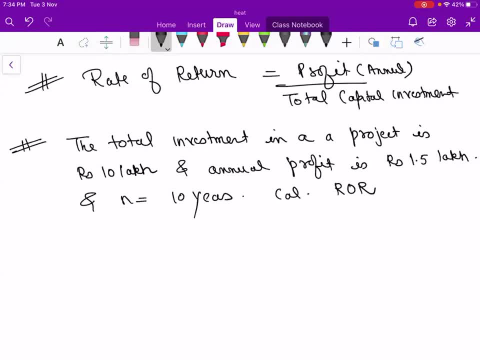 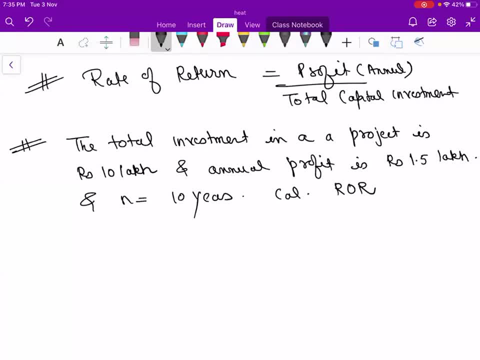 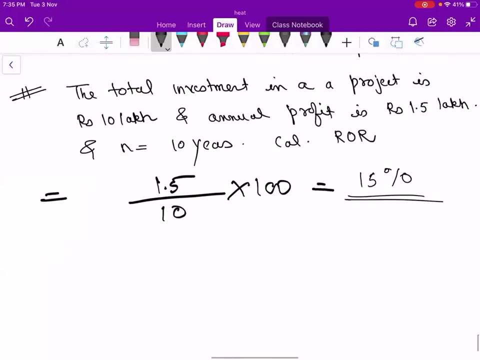 Okay, answer others. please attempt the question. so it will be 1.5 upon 10 into 100. so how much it is coming? 50%, okay, that's it, okay. okay, yes, n equals to 10 is given to confuse. okay, because we had this. ROR is per year. 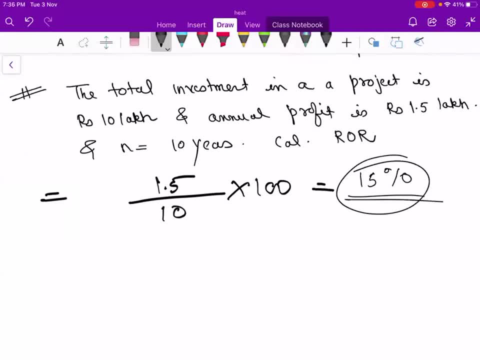 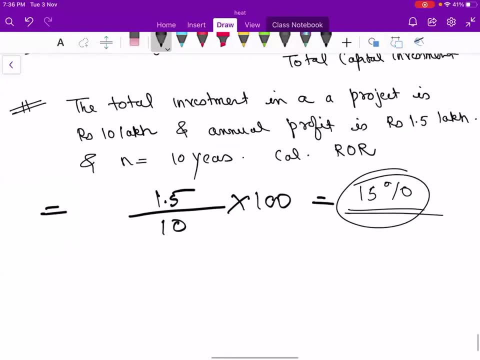 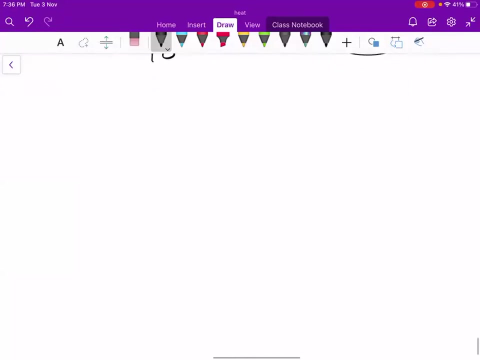 it is not the ROR of the total investment: okay. a total profit: okay. so it's all it's dependent will. they will tell you that, whether you have to calculate in percentage or on that, okay, so don't worry about that, since we are doing for activity of the day, we are just trying to get the 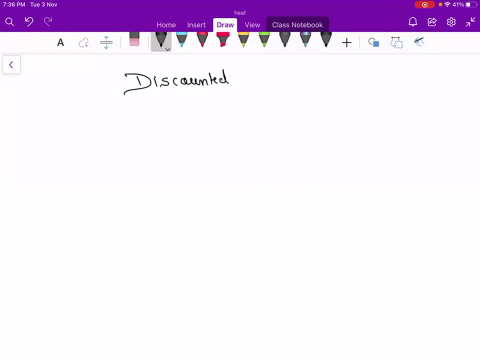 calculation and the total. this will be 0.5, as we have taken as a keyboard PDF as an activity, so that way the RORs no longer get the into 50, 17 Prius, because we now know the original capital cost of gas said 50, 15, 3 저기. 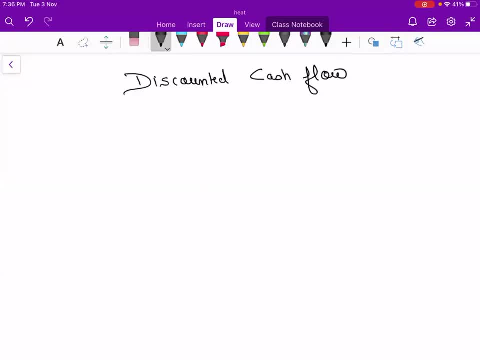 reasonable RORs do 입니다. compounded cash flow is nothing but i effective. okay, just one terminology. suppose you have deposited 100 rupees in the bank. after i effective, you will get. suppose, 200 rupees next year. okay, after one year. this is the value at suppose 2020. and you are getting this value at 2021 by using 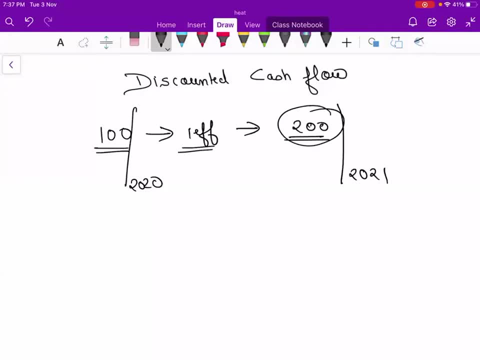 compound interest formula. okay, so if reverse is given, if reverse is given here, so this is known as discounted cash flow- means: how much discount is there for the today's value? okay, how much discount is there for the today's value? it is just like that someone, uh will say to you that 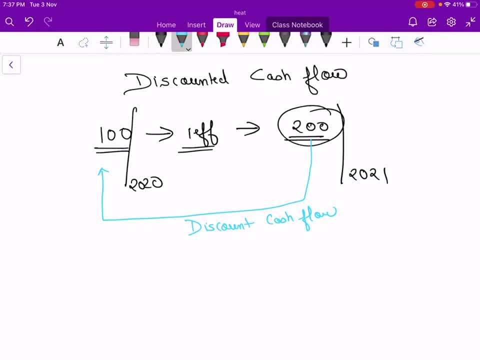 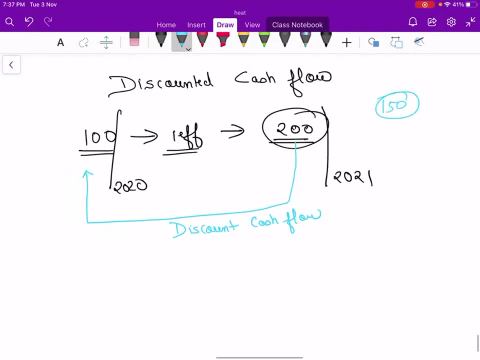 okay, i will take money from you. so you want it today or you want it tomorrow? okay, so you will say that i will. uh, so he will say that i will give you after one year, but the amount is suppose. amount is suppose, uh, 150 rupees. okay, suppose 150 rupees, so it is a loss for you. okay, because the amount is what is. 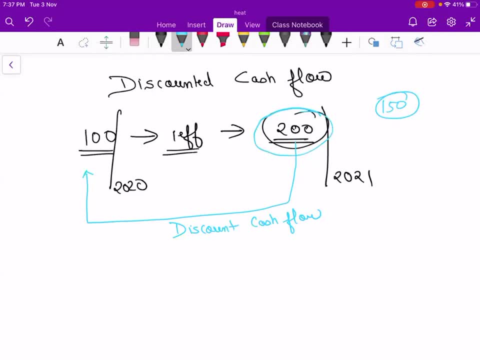 200 tomorrow, okay. so that is what discounted cash flow means. means when you are going, when we are going- 100 to 200 after one year- we use i effective word- okay, and we are going when 200- 200. so that term is known as discount, discounted cash flow. that's it. there is nothing new in that. 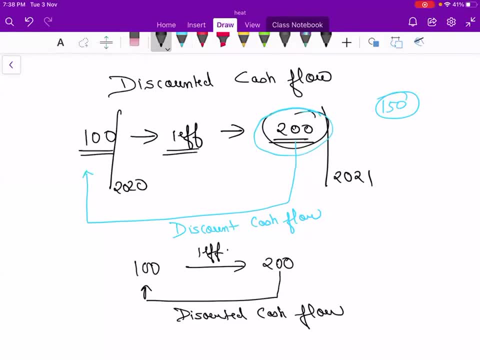 okay, why the word discount word is coming? because there is a discount after one year. it is 200- 200. but you are going from 200- 200 means it is 100 rupees discount. that is why the word is coming: discounted cash flow. there is nothing new in that. okay, okay, okay. so there is nothing new in that, so 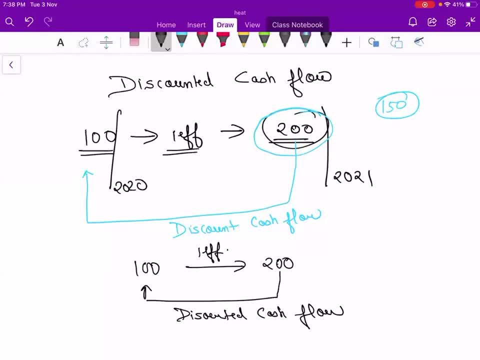 basically, when future amount is going to present amount, so that value- we are uh, saying that it is discounted cash flow, because normally we say that it is i effective- means we are going present to future. okay, here we are comparing future to present, that's it. okay, so the percentage will. 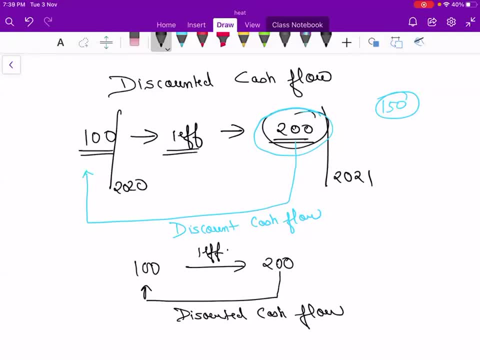 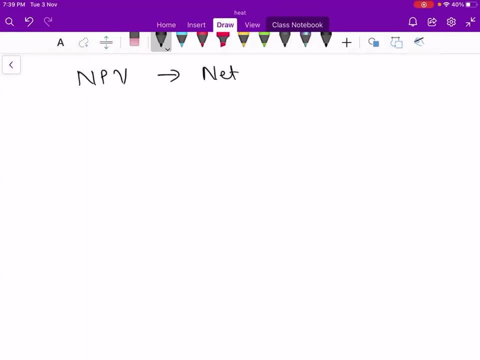 n, n, p, p, p, v, that is v, that is v, that is net present, net present, net present value. what does it actually means, okay, net present. what does it actually means okay, net present. what does it actually means okay, net present value? okay, so it means that suppose today you 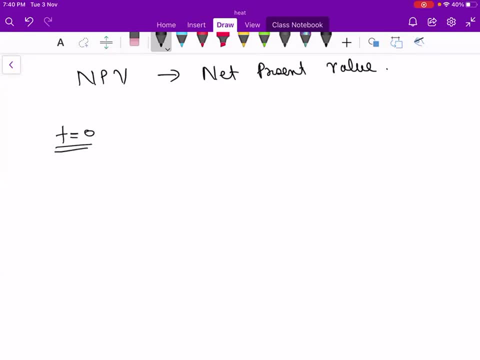 okay. so it means that, suppose today, you okay. so it means that suppose today you decided- decided- decided at time t equals to you, decided to start at time t equals to you, decided to start at time t equals to you, decided to start a industry, a industry, a industry. okay. so it means that suppose today you decided, at time t equals to you, decided to start a industry. 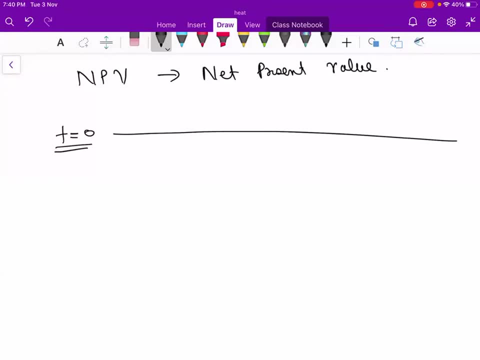 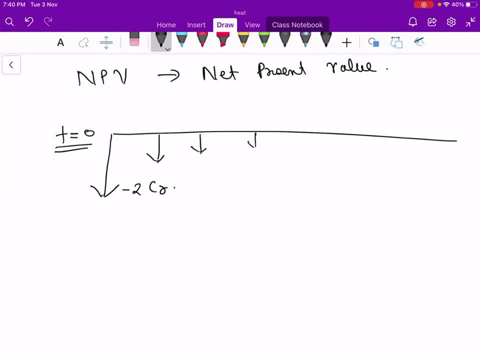 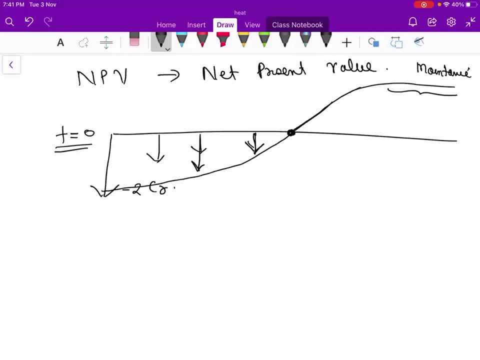 And if that NPV is coming positive, it gives us idea that we have to start that industry. Means you have two options, suppose: okay, You want to start one steel industry business and you want to start some coal industry business. okay, 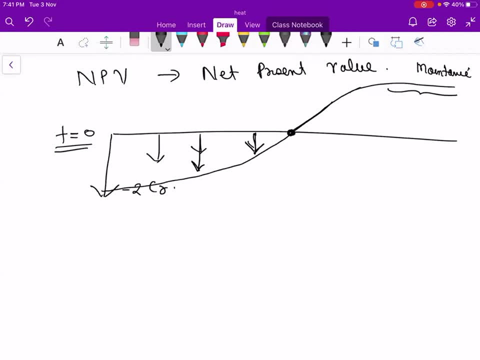 So how you will decide? okay, You will decide that, whether you have to go for steel industry or coal, okay, Basically, this is a profitability analysis method which gives us some rough idea regarding can we start the industry? So how we start the industry. 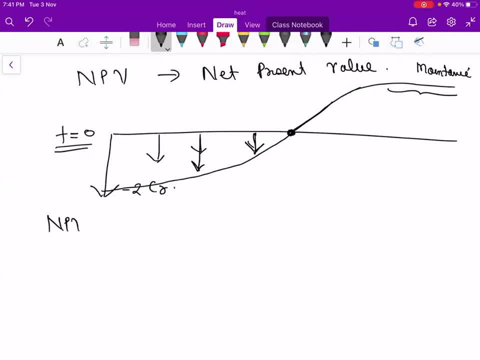 If NPV value comes positive? okay. If NPV values comes positive, it means that industry we have to start. If both are positive, then which one is greater? that industry we will start. okay. So how to calculate the NPV? okay. 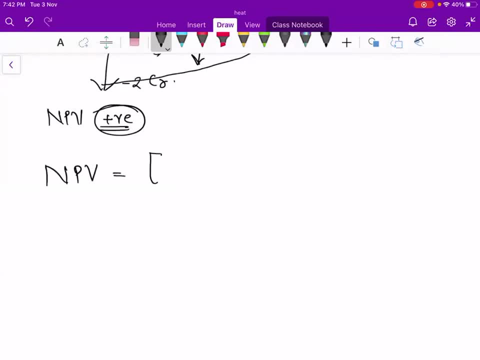 How to calculate the value of NPV. The formula is: P minus E minus D. PD- Okay, 1 minus 5 plus D. okay, Plus D. I will explain each and every term. okay, So in books they have given different notations. 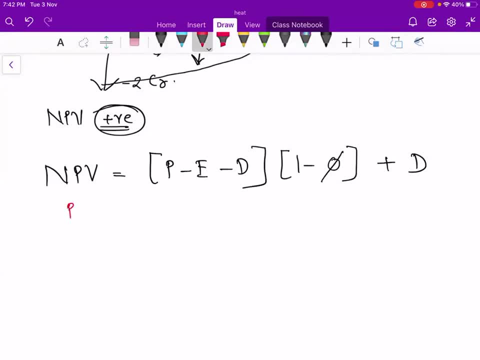 So I have different notations. So here P equals to profit, E equals to expenses, D equals to depreciation, So 5 equals to income tax percentage. okay, So see, here You have a profit of, suppose, 10 lakh, okay. 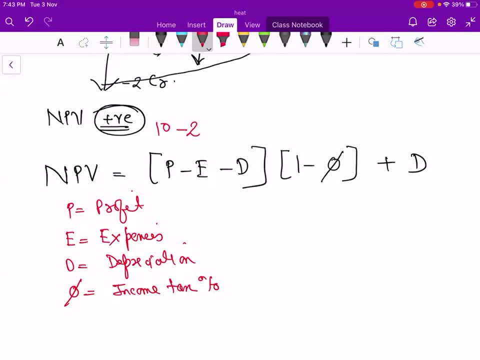 You have a profit of 10 lakh minus your expenses. In expenses it will come your electric bill, your stationary bill and your worker charges, and all that okay, Because that is not your profit actually. okay, wages to the salary to the workers and all that okay. and d means d means depreciation. why we are 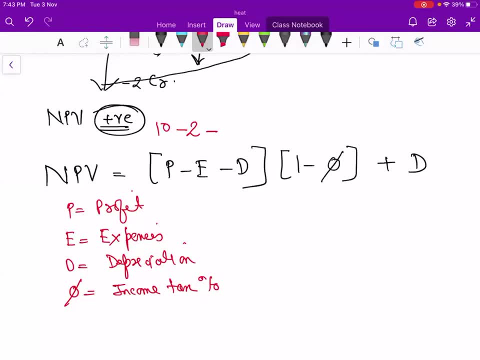 subtracting the depreciation because government says you don't have to in a, you don't have to pay taxes on the depreciated amount. okay, you don't have to pay the tax on the depreciated amount, so the suppose depreciation is one, so it will come on this amount. so how much it is coming? 10 minus. 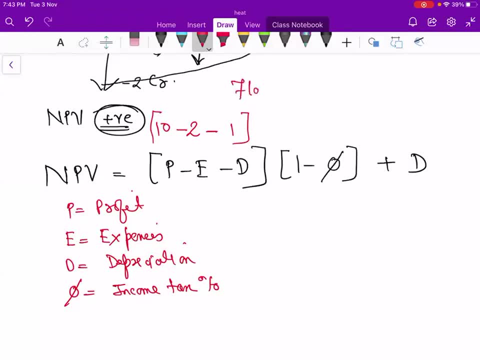 2 minus 1, so it is coming 7 lakh means government says: now you have to pay the income tax on 7 lakh because if you have not subtracted the depreciated amount, this will be greater value. it will not be 7 lakh. what it will come, it will be 8 lakh. so suppose this percentage is 20 percent. so which? 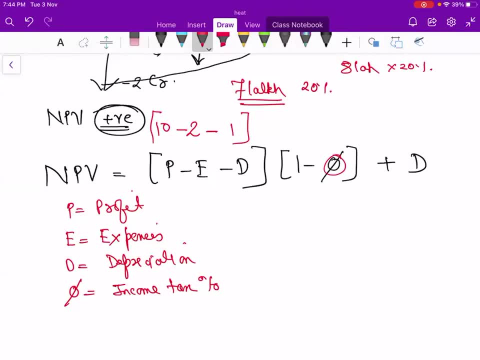 one is greater: 8 lakh of 20 percent will be greater, or 70, 7 lakh of 20 percent will be greater, or obviously 8 lakh of 20 percent will be greater. so that is why we have to, i have told while teaching the depreciation. also, the government says you don't have to pay the taxes on the. 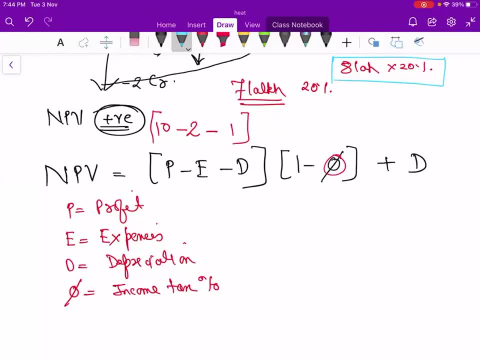 depreciated amount. so this is 10 minus 2 minus 1, this is 1 minus 5. you take it 20 percent point to 0. okay, but for us it is not depreciation amount. okay, we have seen that for us there is no depreciation. that is why we have to again add that one value, okay? so this is what is. 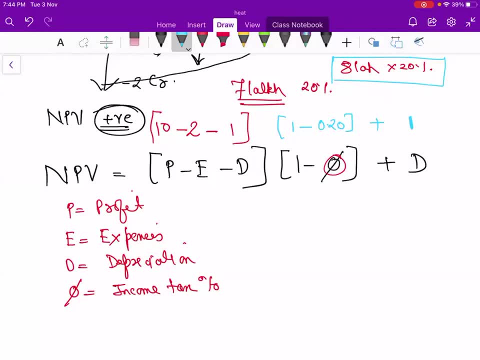 this value. okay, what is this value? okay, this is known as: okay- wait, i will don't write it npv here. better word will be acf- annual cash flow. okay, this is annual cash flow. okay, what is annual cash flow? i am explaining once again. listen carefully. okay, annual cash flow basically means p minus e minus. 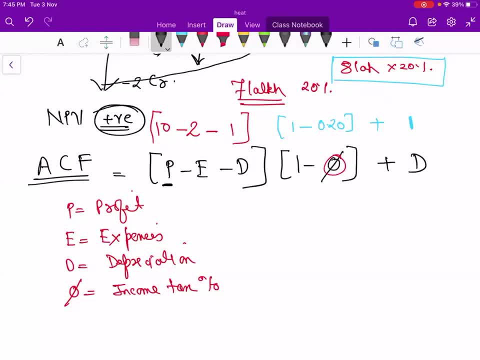 d, 1 minus 5 plus d, what is p? profit means you are running an industry and you are getting a profit of 10 lakhs. okay, i have taken 10 lakh minus expenses. what is expenses? your electric bill, your salary to your workers? okay, your contingency bills? okay, that minus we have done. 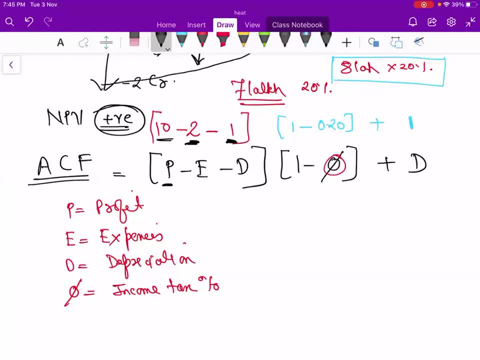 minus one depreciated amount. we have done. why we have done the depreciation amount minus? because government says you don't have to pay the taxes on the depreciated amount. so we have seen when we minus subtracted that depreciated amount it gives us profit. okay, why? because 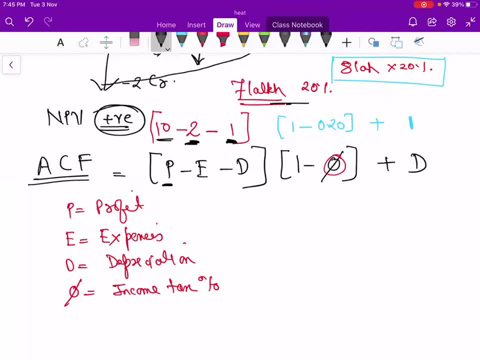 if we have not subtracted it is coming eight lakh, so eight lakh of 20 percent. you have to pay more income tax. so now, after depreciation, it will come seven lakh of twenty percent. so you have to, uh, you have to, you have to uh reduce your, uh, uh, that problem, sorry, you have. 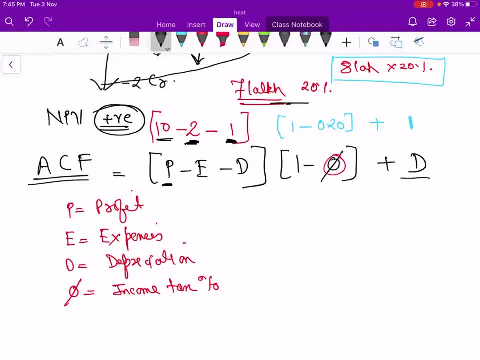 to reduce the income tax. okay, it means it gives a profit plus d. at last you have to add d because for us it is not depreciated. okay, so this is annual cash flow. okay, what is this? this is annual cash flow, or you can say actual profit to my system. okay, this is. 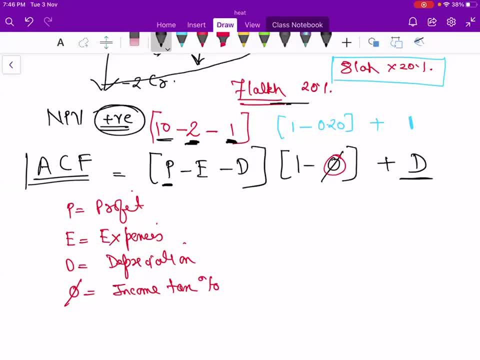 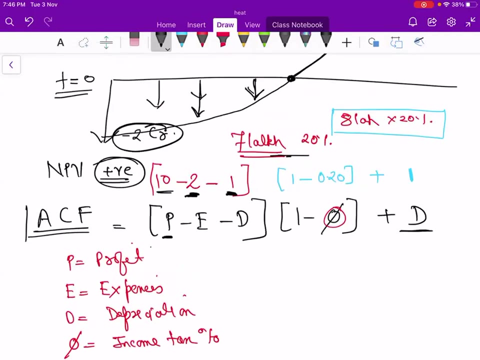 annual cash flow. okay, so this is. annual cash flow means actual profit. that means we can say: this much amount i am getting every year. okay, so it means that suppose here it is two crore rupees, so every year how much i am getting. if i calculate this value, this much amount i am getting every year. 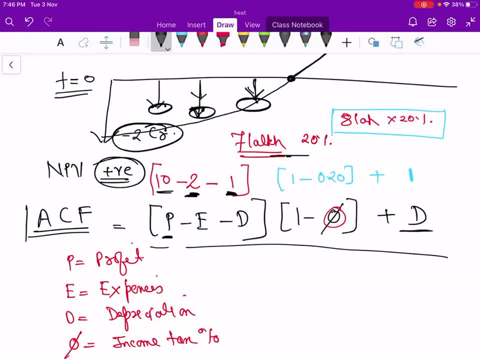 okay, this much amount of money i will be getting every year. so everyone got this point. annual cash: okay, i will explain npv first. annual cash flow: everyone got this point. yes, annual cash flow: you can say it is the total amount which i am getting from my business. 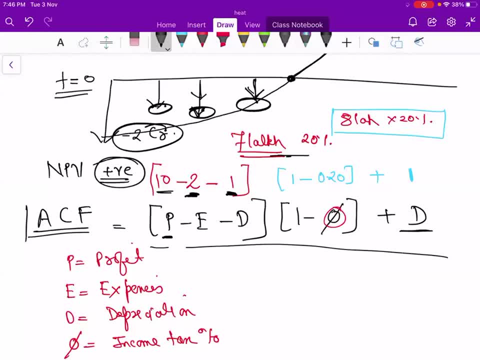 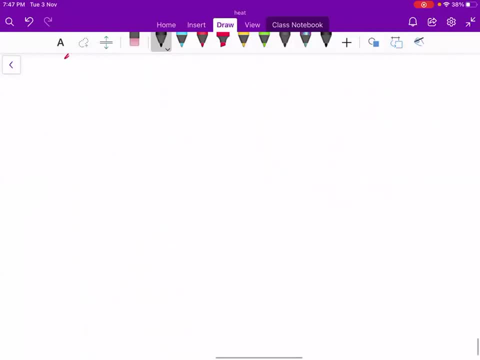 okay, every year. yes, it will be every year. annual cash flow will be every year this much amount you are getting from your business every year. so now i want to calculate the annual cash flow: NPV net present value. okay, now I want to calculate NPV net present value, so it will be always at. 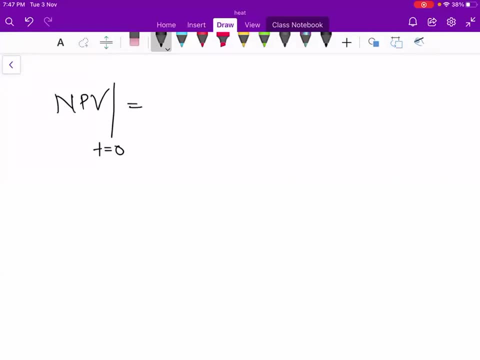 time t equals to zero. so how much I have invested, how much I have invested at time t equals to zero minus two crore. so what NPV will come? okay, NPV will come minus two crore, plus after one year there will be profit. okay, I have invested two crore rupees. now there will be the profit from. 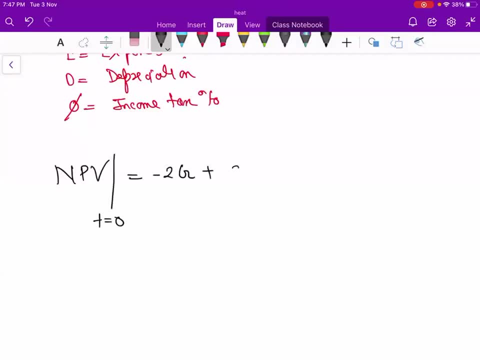 the second year how much profit I will be getting. suppose something x value. suppose something x value, I am getting profit. okay, so this x is one. this I have to come back because I have to calculate. at time t equals to zero. so what will be the formula one plus i to the power one will come. 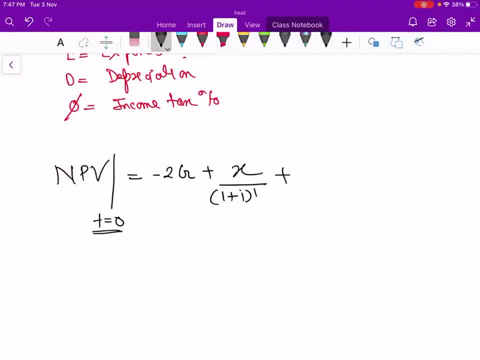 plus. if ACF is same for that year, okay, then it is suppose it is different. y equals to one plus i. how much here I have to come back two plus z upon one plus i to the power three, up to who can say any value, it will come okay. so this: 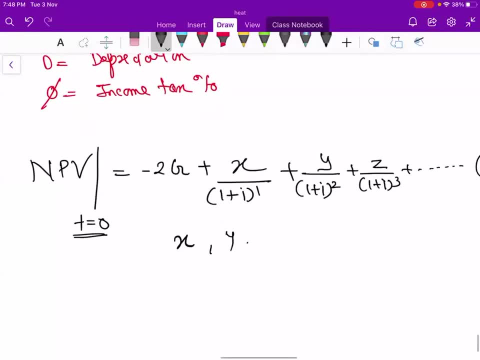 x YZ, this X YZ may or may not be same. may or may not be same. okay, suppose if it is same. okay, yes, Y, Z are annual cash flow. Suppose this ACF, this is ACF. okay, Suppose if X equals to: 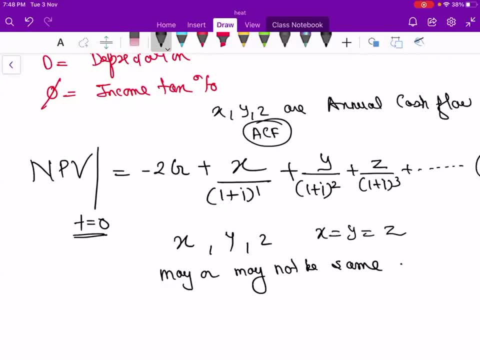 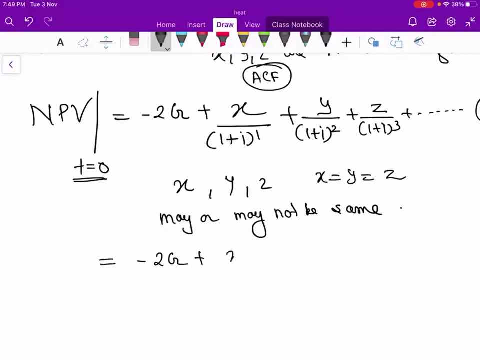 Y equals to Z, which formula I can use here? If X equals to Y equals to Z, which formula I can use here? Annuity, Very good, Okay, So it will be annuity formula I can use. Okay, So it will be minus 2 crore plus X, 1 plus I to the power N minus 1 upon I, 1 plus I. 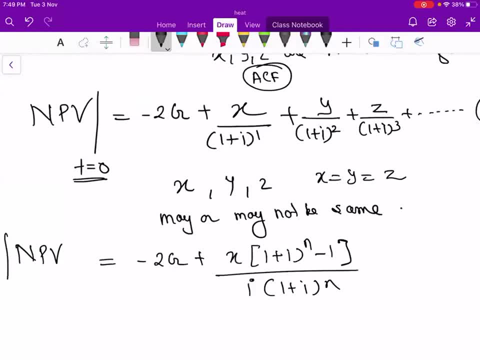 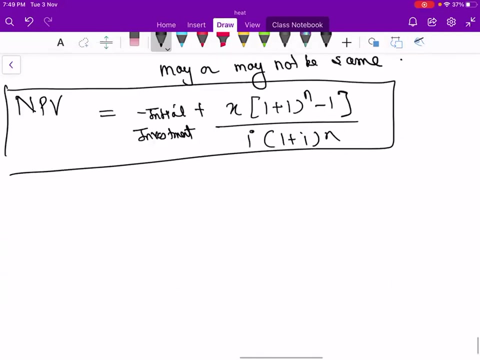 to the power N. So this is NPV. Okay, This is NPV. So, in generalized word, if you want to write here, don't write at 2 crore, write it. initial investment, Initial investment. Okay, So everyone got this point. Okay, This is investment. I will explain ACF once again. 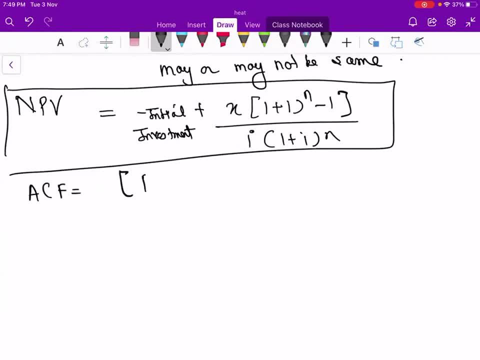 See what is ACF. ACF equals to P. P is profit minus expenses, minus depreciation. 1 minus 5 plus D. Okay, So this will give me an. ACF means actual profit to my industry, Okay. Yes, Initial investment will be negative sign. Okay, Because at that time you are in the 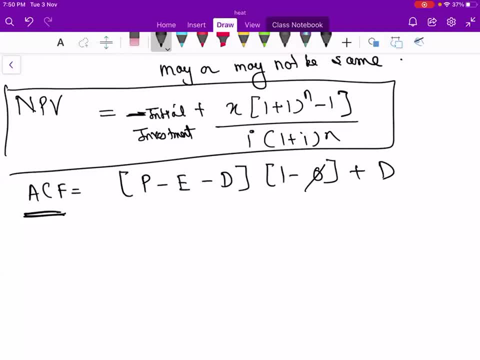 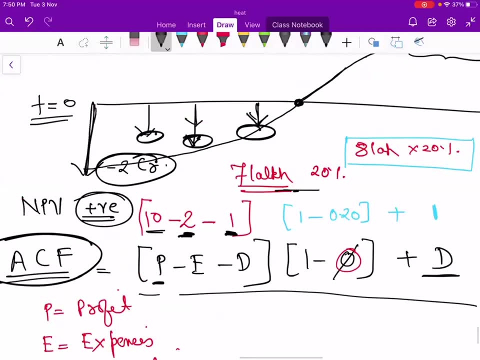 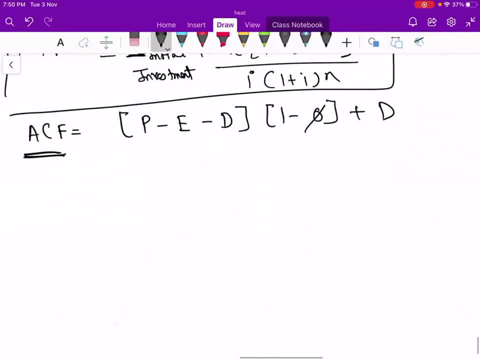 loss: Okay. Initial investment with negative sign: it will come. Okay. That's why I've written here: minus 2 crore. Why See here? Because you are in loss actually. Okay, This 2 crore污 has gone from your pocket. Okay, This 2 crore s is gone from your pocket, Okay. 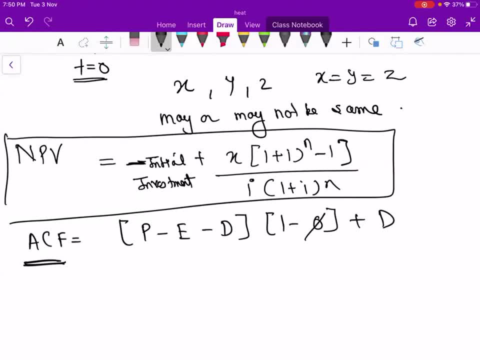 That is the thing. Okay, Everyone understood. Everyone is comfortable. ACF is annual cash flow. See this formula. I will explain once again. Don't worry about that. Okay, But see this formula. See all the things which I have written here. 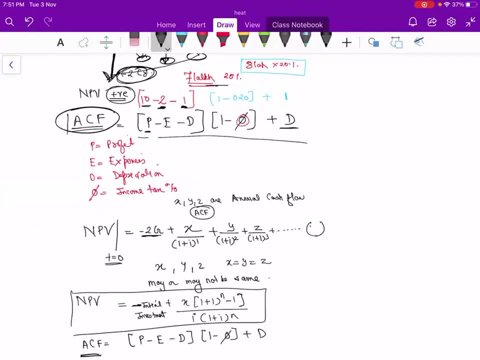 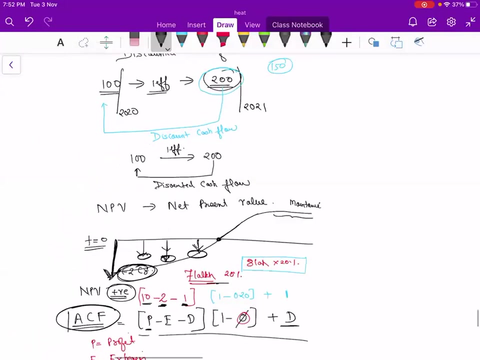 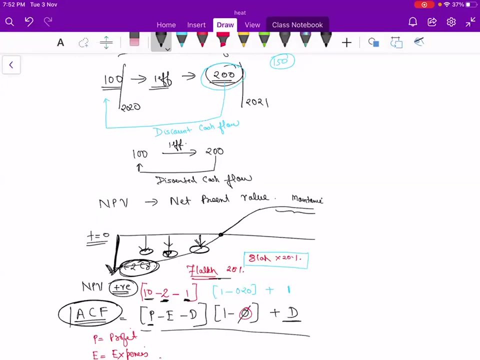 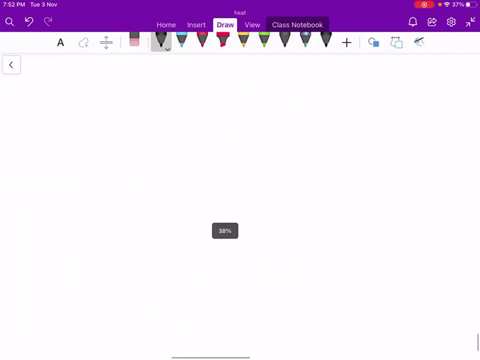 Okay, I will explain once again. Don't worry, We will solve question on this topic tomorrow. So everyone is comfortable, Everyone, Okay. So I will explain once again all the terminology. Okay, Listen, What is NPV? 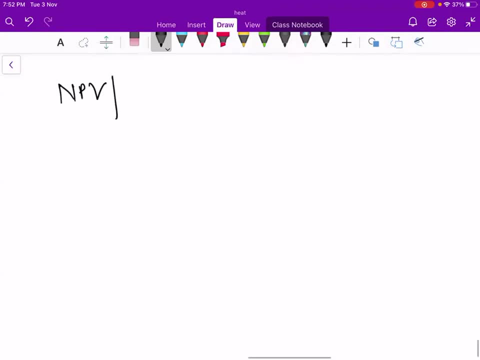 NPV is net present value Means all the values we are calculating at time. t equals to zero Means basically what we are doing. Suppose before starting the industry we have calculated that, Okay, We need a 2 crore rupees for starting the plant. 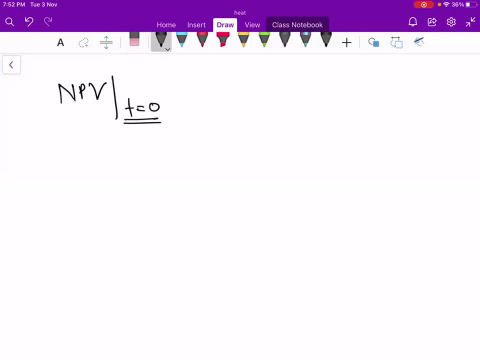 Okay, So what product you are making, you know that. Then on the basis of that, you will see that what is the cost of that product in the market, At what price you will sell that product. So, actual profit, how much you will get. 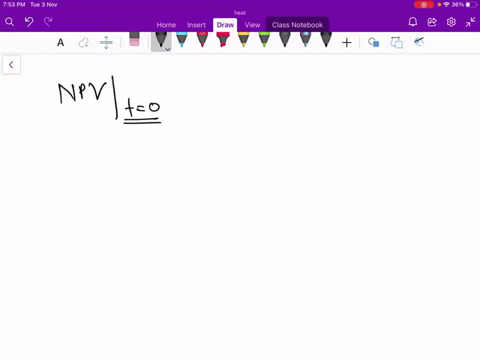 You have income tax value. You know how much value is depreciated, All the things you will calculate for your industry. Okay. So on the basis of that you will select. Okay, I will go for this industry. Okay, So that is why ACF. you will calculate that NPV should be higher. 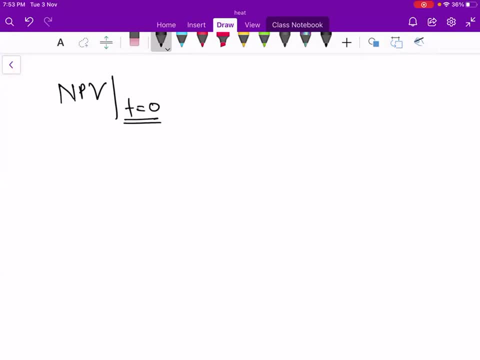 The industry which NPV is higher means. basically, it means that which industry will give you more profit, that industry you will select. Okay, So for NPV, we know that we should calculate first the ACF value. So what is ACF? 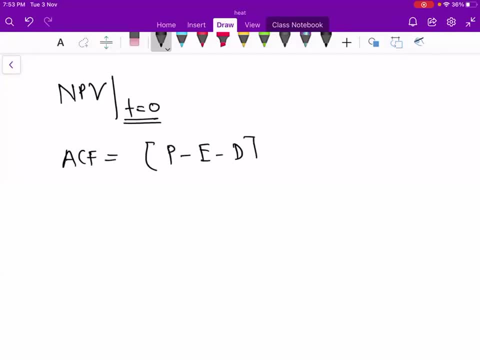 ACF formula is: P minus E minus D, 1 minus 5 plus D. Okay, So means I will give you an example. Suppose your profit is coming every year is 20 lakh. Okay, Minus expenses, 5 lakh. 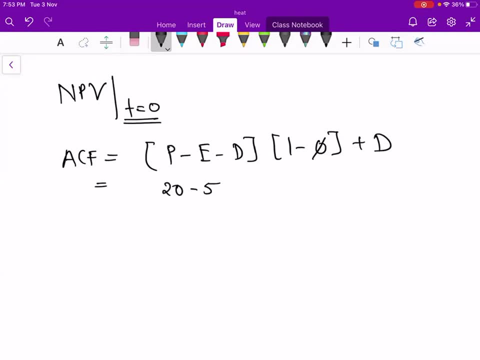 What are expenses? It can be electricity bill, It can be contingency bill, It can be the money for your raw material, It can be the money for your salary to your workers, anything Okay, So that obviously that is not your profit. 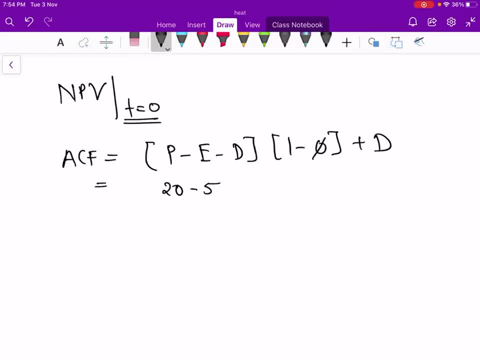 Okay Means basically: Suppose you are running a small shop. Okay, At the end of the day, at the end of the day, you got 20,000 rupees in that system. Okay, In your bank, suppose you got 20,000.. 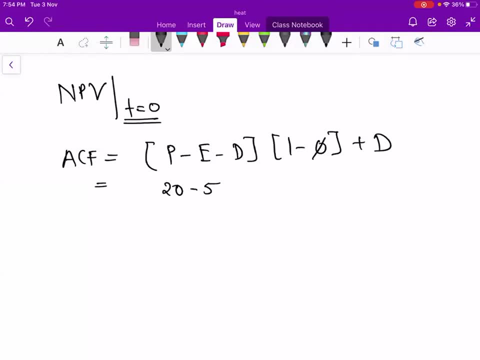 So is it 20,000? is your total profit that you will take home? No, From that 20,000, you have to give the electricity bill, You have to give the money to a sweeper, You have to give the money to the boy who is working, the person who is working in your 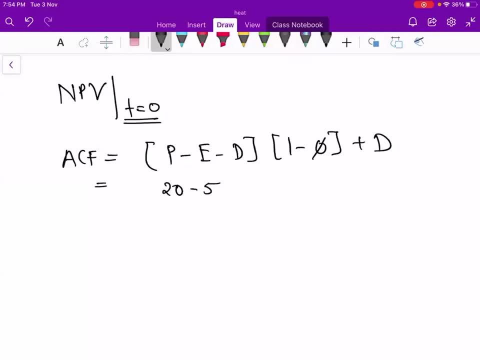 shop. Okay, You have to pay the charge- This of the, that thing, that any contingency, anything- Okay, You have to pay. after that, You have to pay the income tax to the government. That is, we pay in the terms of a GST. 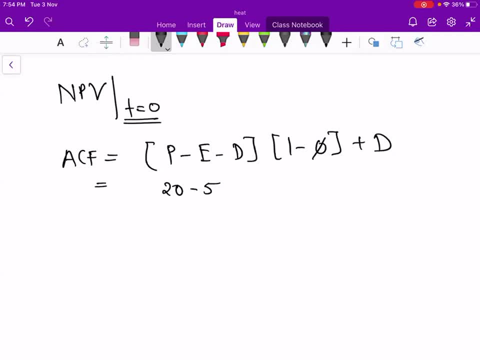 Okay, VAT: You have seen that we pay tax on the debt terms also. Okay, So everything you have to pay. So that is minus expenses. Okay, So in expenses only, we are taking about the salary, raw material and all that. 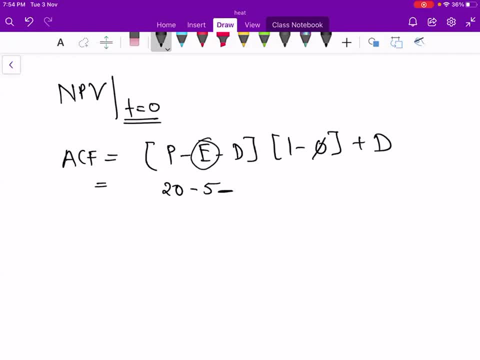 Minus depreciation, which we are doing, What is the depreciated amount? The object, the money, the equipments which you have Purchased? now it has of low value. Okay, So that you have to decrease, Suppose one. you have reduced it. 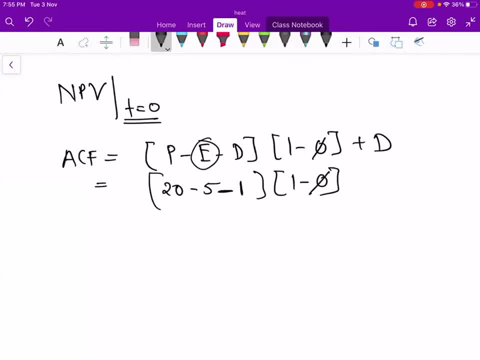 So on that value, one minus five. So you that five is income tax. You are paying to the government plus depreciation. That is one you have to do, Okay. So basically what it, what this formula is giving this value is giving the money after income tax, money after income tax plus depreciation. 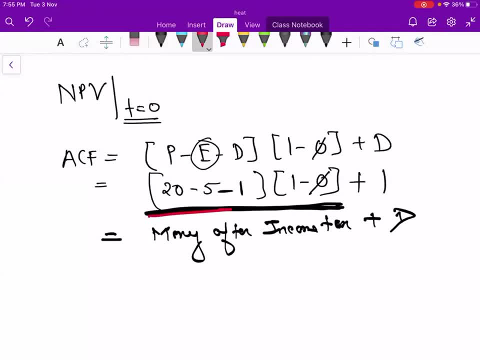 Okay. This red line is basically the money after income tax, plus in that you have to apply the depreciation, Okay, Okay. So that is the thing. after every expenses you have to pay, the means profit will come Now. NPV. 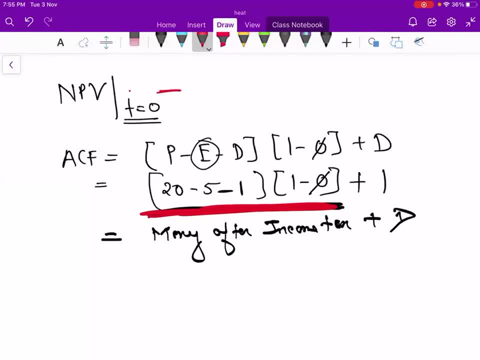 Okay, So in the initial investment you have done, suppose two crore rupees, So it will be minus two crore Plus every year. if ACF is coming, then ACF upon. if it is only one year, then one plus i to the power n only one year.